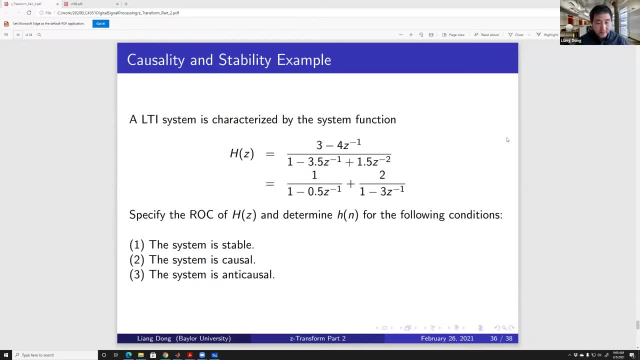 Good morning class. Let me start with what we had last time on the quiz problem. So here is the problem. Last time we work on it, we define an LTI system using its system function, which is the impulse response H in the Z domain. we call that system response or system function. 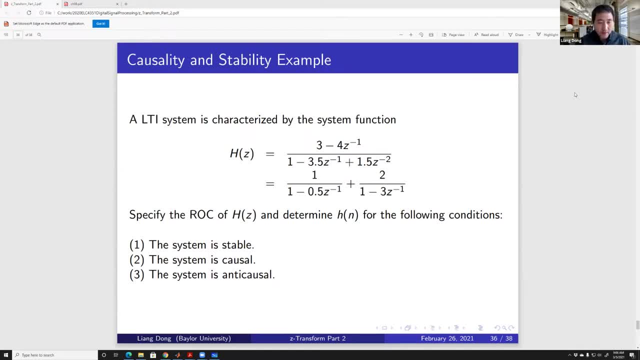 So this system function is in a rational format. because it's LTI system, We got this numerator denominator. both are in the polynomial term, That's a polynomial of a variable, Z, or variable of Z to the power, negative one. Conventionally we like to use Z to the power. 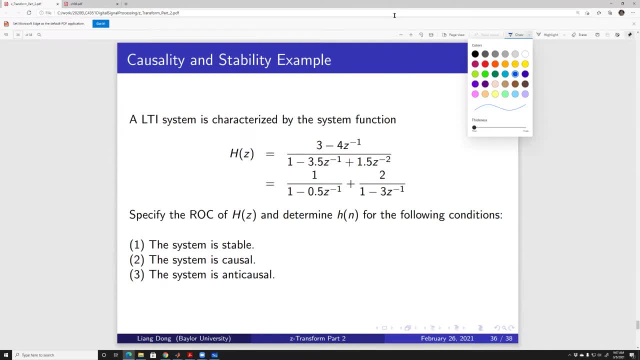 negative one because it's easy for me to transfer back to the time domain. Okay, so anyways, we want to specify the region of convergence of HZ and then determine HN doing an inverse Z transform of the following conditions: The system is stable, the system is causal, the system is anti-causal. So first we 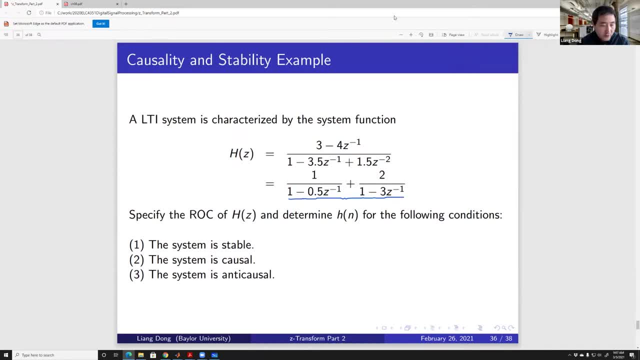 examine here. this is the partial fraction expansion We end up in. this is last step. So we find out there are two poles for the system function. P1 is equal to 0.5, which makes first term equal to zero. right P2 is equal to three, make the second term equal to zero. on the 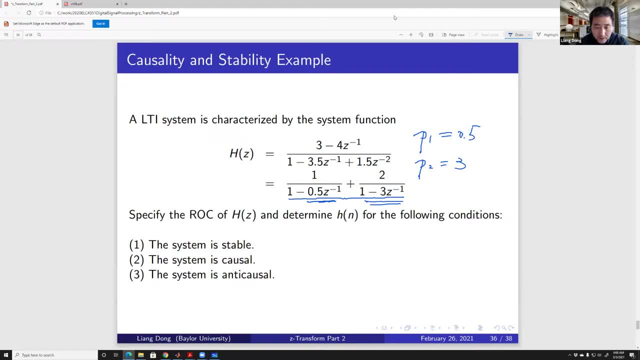 denominator. So those are the two poles. Now, because it's a function of Z to the power negative one, therefore, I simply using 0.5, you can, you can kind of copy this coefficient 0.5 and this three. 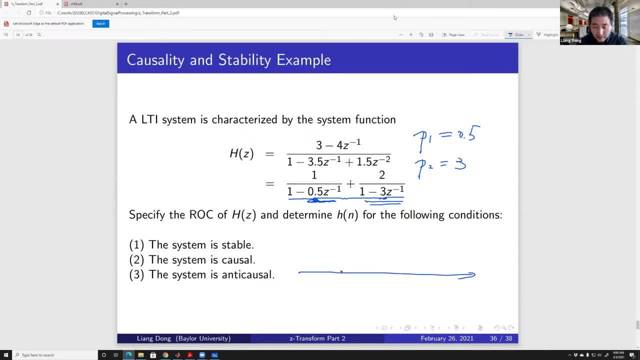 So I have on my Z plane. this is imaginary part, This is Z plane real part. I got two poles: One is here, 0.5, and then there's one, two, three, another is here three, 0.5. Those are real poles And we we know for the region of convergence. 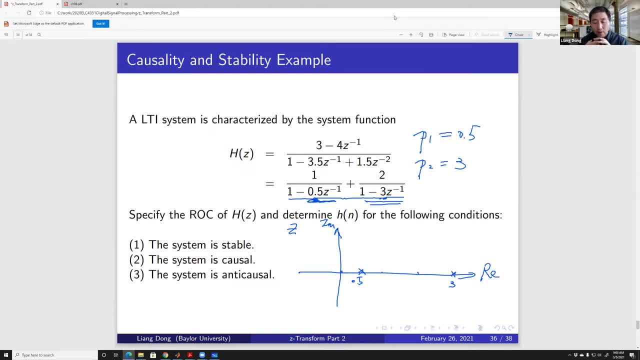 it is a, it is a circle. The shape is a circle around the origin. So we let's just plot out this circle. That's a, a round 0.5 cross 0.5, and then a large circle cross three. 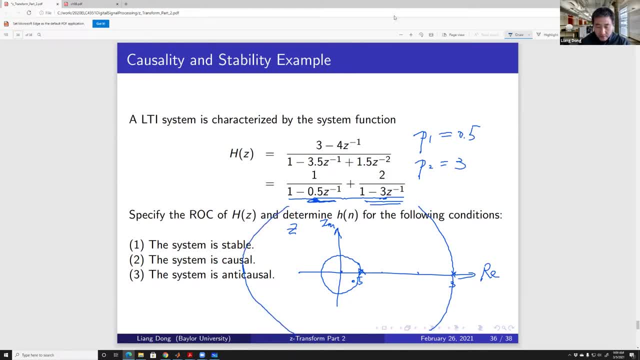 This is over here. It's cross three. And then we also want to plot out the unit circle which is right here. That is the unit circle where I got a one here Right. So the system is stable. We said, if the system is stable that I will have to get this unit circle within the region of convergence. 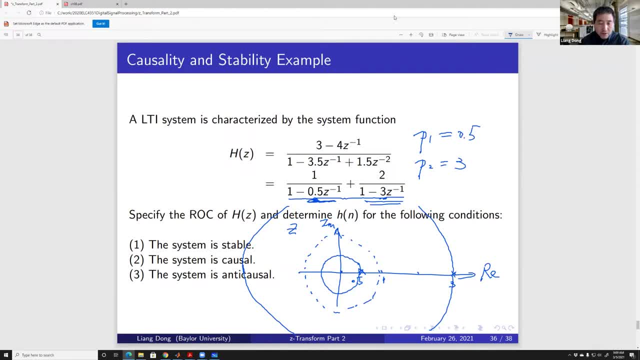 The reason being that only the unit circle actually makes physical sense. Whenever I need to check the signal in the frequency domain, I am taking z equals to e to the power j, omega, or in another word, I'm taking z absolute value equal to one, So I'm not going to look at its 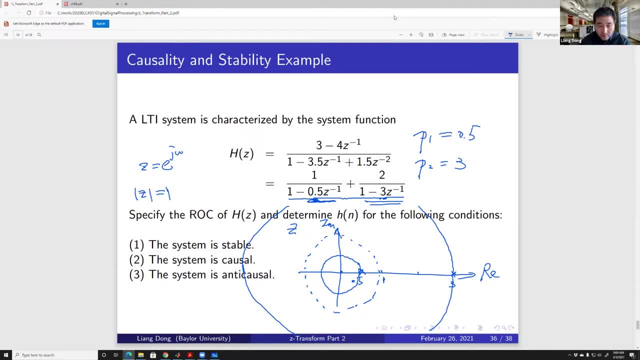 amplitude. I'm only going to look at its phase j, on j to the power e, to the power j, omega. So I am travel along this unit circle in this direction And that is my frequency from zero. This is frequency from zero to pi over two, to pi, three pi over two and back to two pi And, of course, 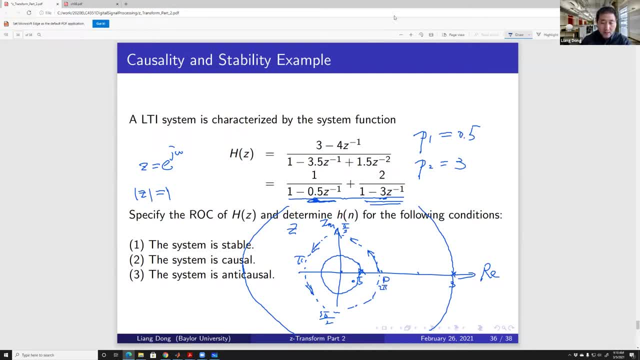 we know, because everything this is this discrete times signal. so pi, this is the highest frequency i can have, which corresponding to fs over two. what is fs? that's a sampling frequency. right, that's a sampling frequency. so when i get back it's fs. this is the highest. that's not crystal rate if it's over two, corresponding to 180 degree. 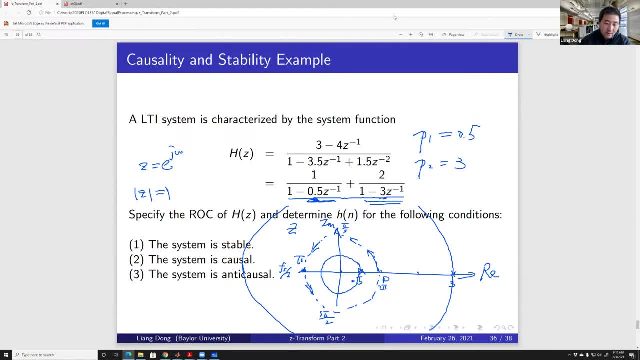 or pi. so i need to make sense that this unit circle will always be converging because the system is stable. so for all the frequency part, the unit circle is safe. the unit circle should be in the region of convergence. so if i'm looking at this picture, i know the region of convergence. 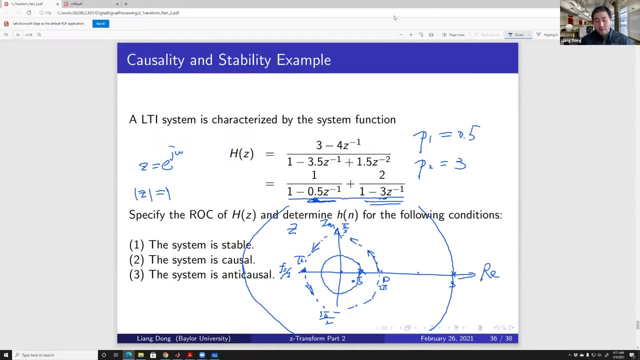 is either in interior or exterior of circle, and those those circles are bounded by the radian 0.5 and the radius 3, because these are the two poles. therefore, for the first problem, the radian convergence is, that is, within those two boundaries. right, but within those two boundaries. 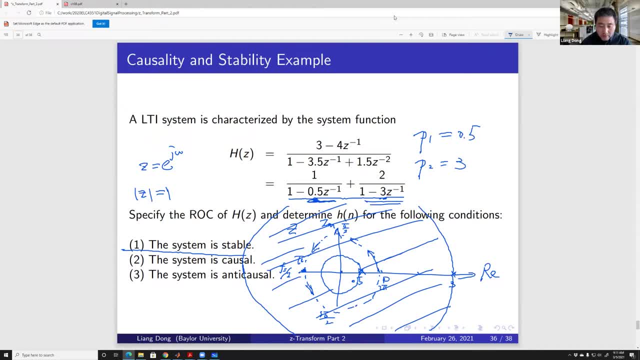 to make sure that this unit circle is in the region of convergence. so the boundary is between 0.5 and a 3. therefore, for the first problem, the region of convergence, is this: okay, less than three. now do i need to use less than equal to less than equal to all? this is fine, less. 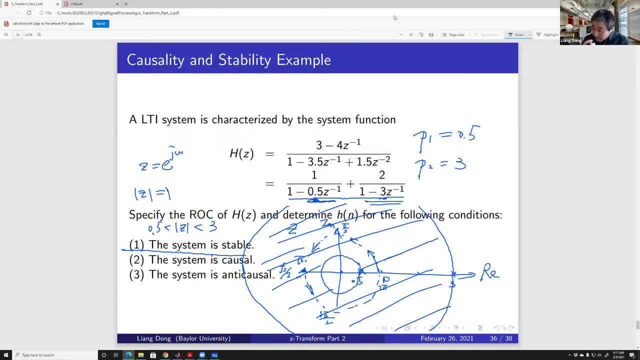 0.5, less than z, absolute value, less than three and of course, i need to use strictly less than right, because you know this point. this point is the pole. the pole is not in the region convergence. so when you're talking about region convergence, you have to explore this pole, so it should not. 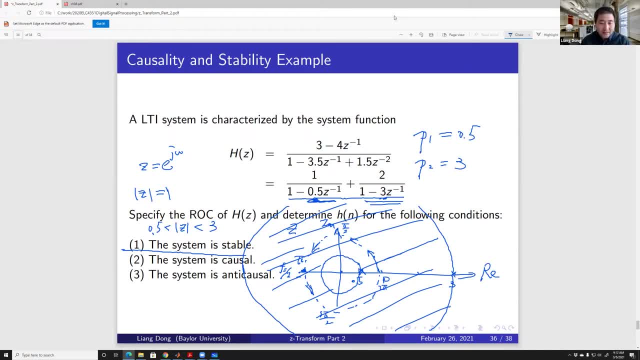 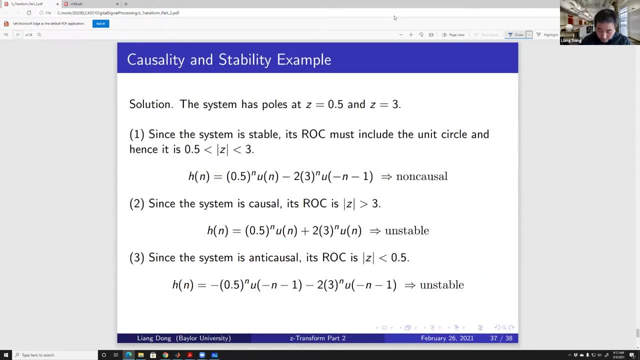 include it. you need to use a strictly less than sign here. so this is, this is okay, all right. so for this problem we will see. the solution is we said i have two poles, 0.5 and a 3 for the first problem, since the system is stable, its region of. 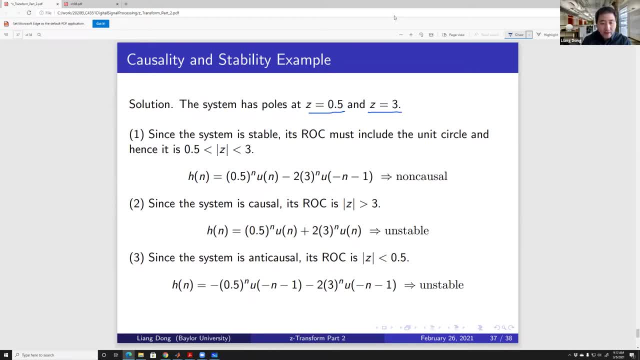 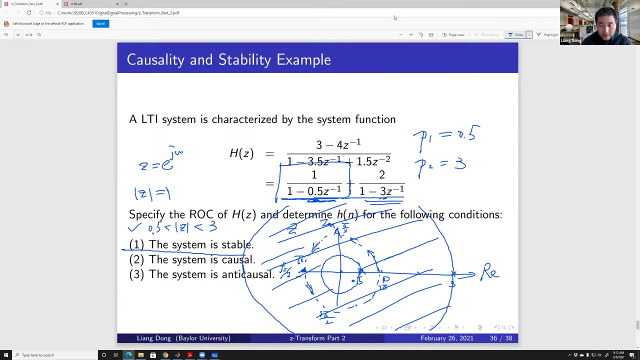 convergence must include the unit circle and hence we have this inequality expression here. then for each part, But the first part. what I meant is this part here. If you look at this part, I got a pole 0.5. And you have this region convergence exterior of this pole. 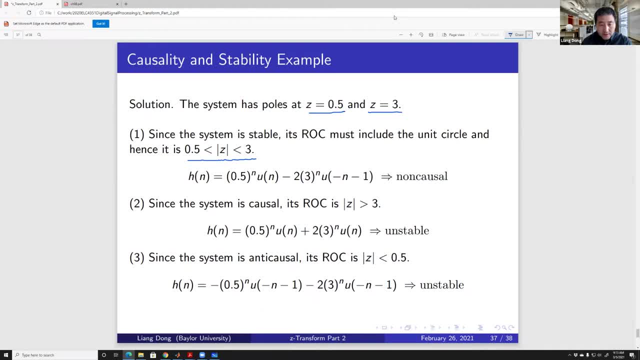 Circle crossing that pole. therefore, the first part, doing inverse, e transform. I'm taking this format which, for the first part only, that's the causal format. causal is region, convergence is exterior of a circle. So you got 0.5 to the power n, u, n. 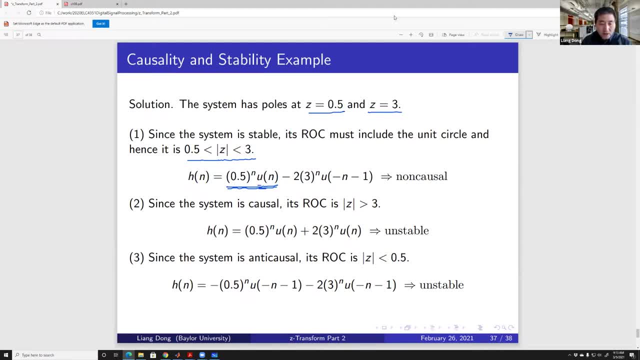 It's very easy to remember that Because Collo system, we put a step function u n, 0.5, that's the root or the base of this- to the power n, this term and this root corresponding to the pole, we got a pole 0.5.. 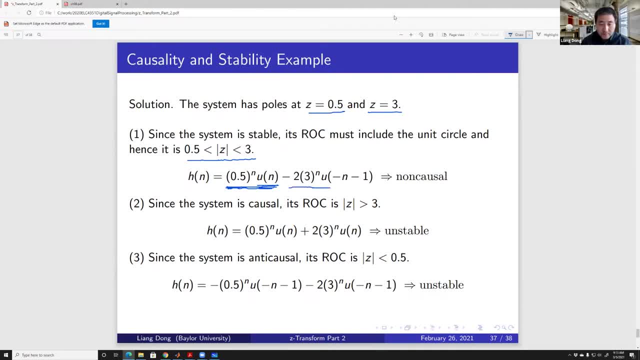 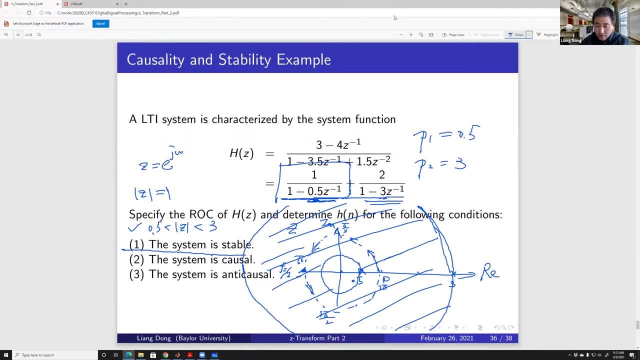 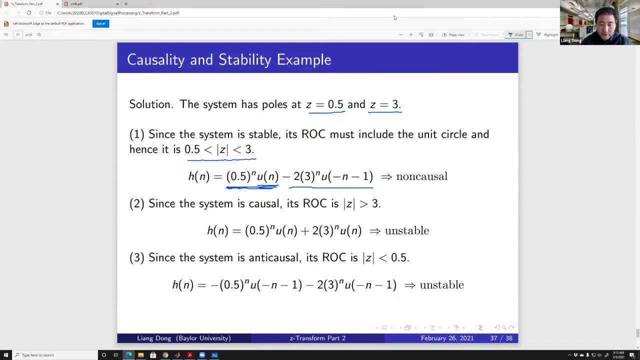 So it's right here. The second term now for this case. for this case that's within The circle that cross points of three radians three. therefore it's anti-collar. the second part. So we put a u negative n subtract one here. 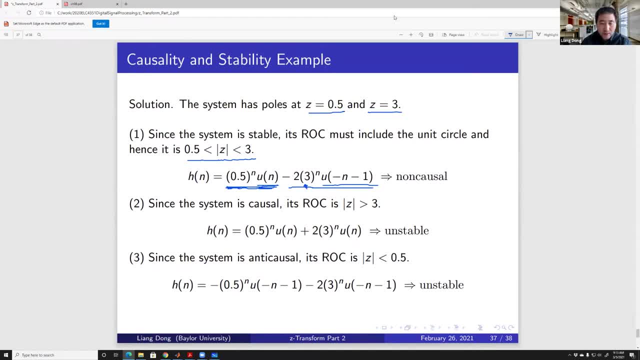 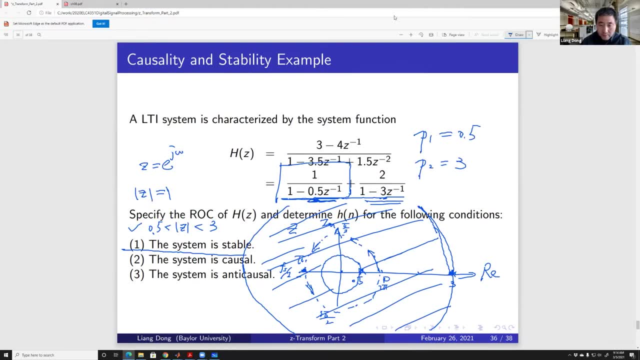 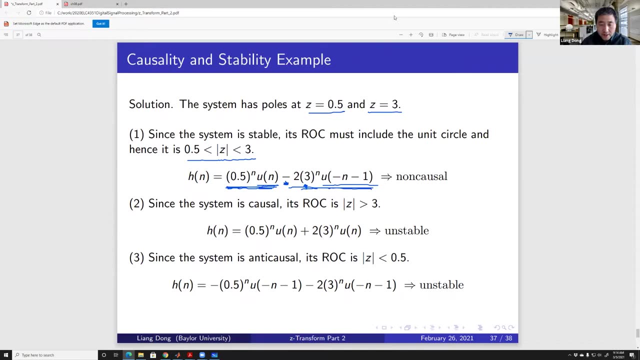 And then again, three is the pole, that's the root. So three to the power n And we are putting negative two here, whereas does the two come account twist, come coming from here. A negative sign is along with when you're dealing with a non-colloidal segment. 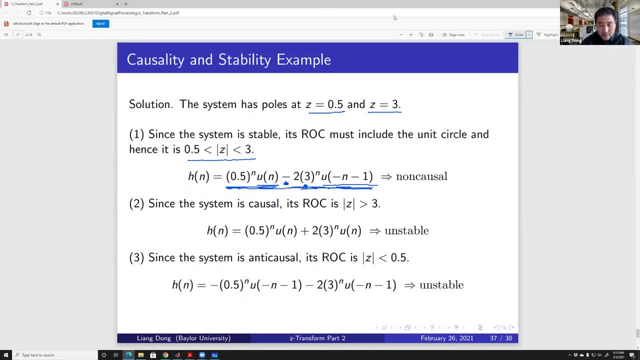 Signal. you will have a negative sign here. Therefore, the final answer is this: Well, this is non-causal. If you're putting all these together, it's non-causal because you got the second term. You got the second term. It's non-causal. 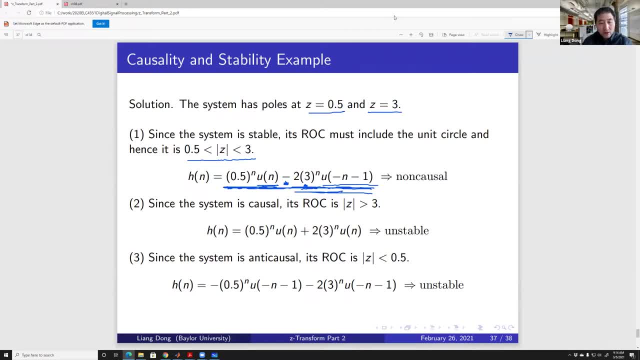 The overall h? n or the overall system is non-causal. The second problem is if the system is causal. if the system causal, then the region of convergence has to be exterior of anything and go all the way beyond, to infinity. Therefore we have to make sure that is greater than three. 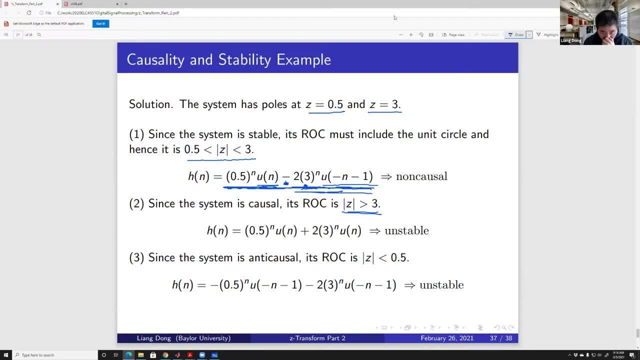 It just the entire exterior thing. So the region of convergence is Z greater than three. And then remember that's strictly greater than that We're not going to include. it's not greater or equal to, because three is a pole region of convergence: exclude, exclude that one. 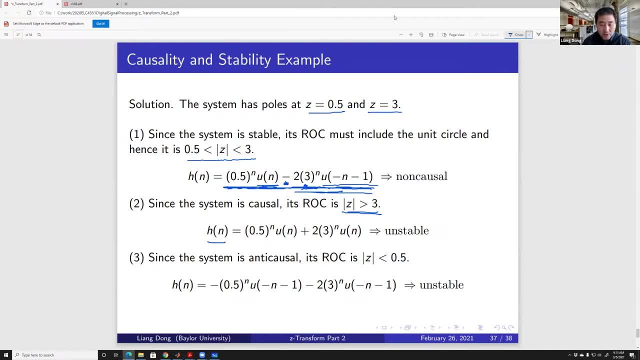 And then h? n can be easily calculated. So we got the first part is causal, second part is causal, So we use both part of u n. Then the entire thing is unstable, Unstable. Why is unstable? Well, because the unit circle now, in this case, is not in the region of convergence right. 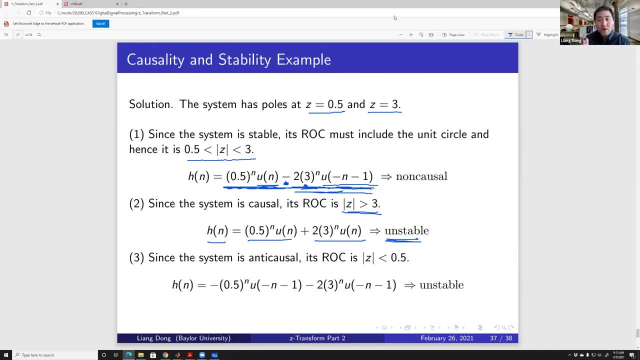 Only the unit circle makes sense because those are the frequencies I'm going to work of practical system along the unit circle. Now, unit circle is not in the region of convergence, So it's not a good system, It's unstable. The third problem is if the system is anti-causal. 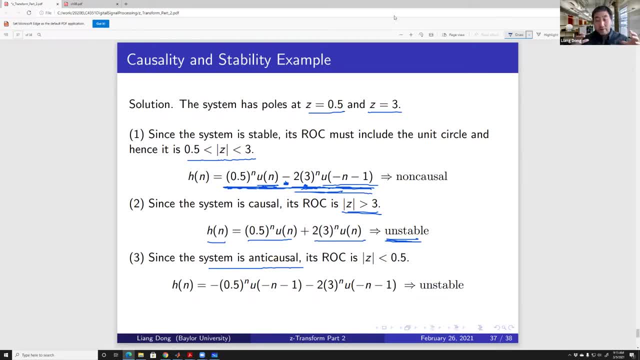 So I know the entire thing is anti-causal. Therefore, region of convergence is integral. This is interior of circle and including the origin. So the region of convergence is Z, strictly less than 0.5, less than the radiance defined by the first point. 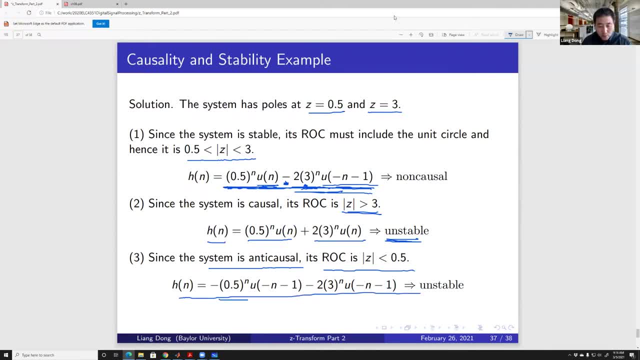 And h n can be written as this: Well, those two parts are anti-causal, anti-causal. So we have this step function here. step function here of n negative n minus one. We got negative sign here. negative sign here. Okay. 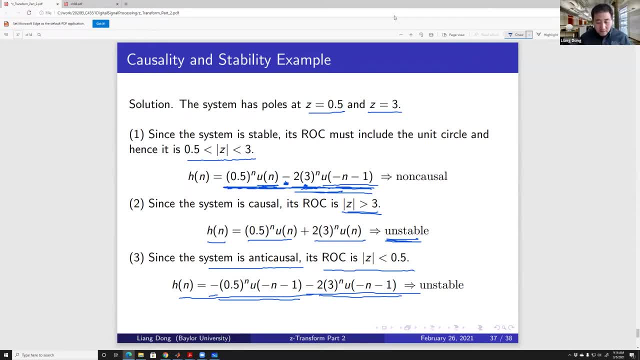 Okay, So what we're doing is unstable because, again, the unit circle is not in the region of convergence. So that's the solution for this problem. So for this problem we were kind of doing an exercise. first We trying to understand region of convergence in a pose. 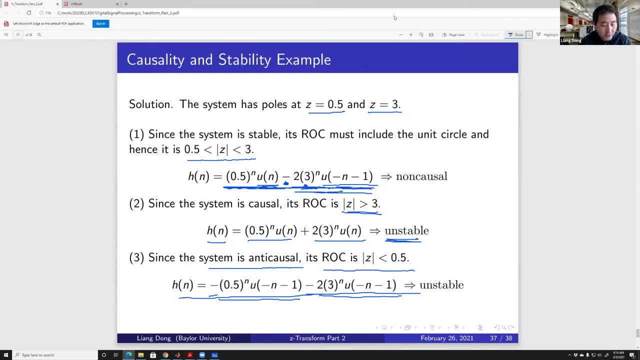 Of course, by definition, pole should not be in the region of convergence. And then we also from this problem. we kind of understand that um by given different regions of convergence. Okay, The final answer for the system: h: n can have different formats, can have different forms. 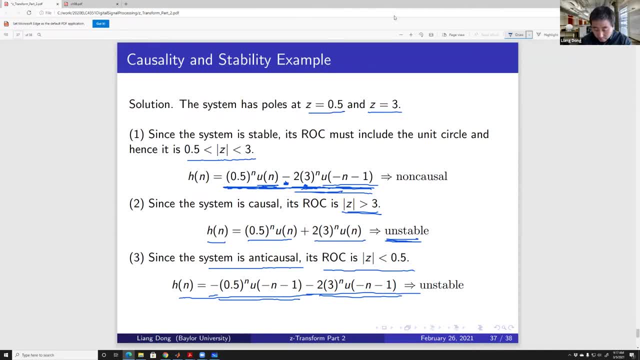 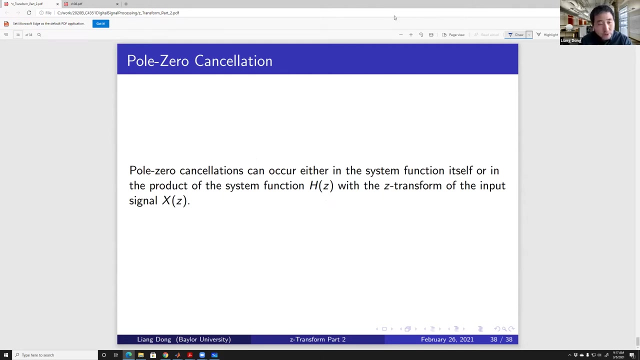 here. I got three different answers and those answers will define non-causal system, unstable system. If it's stable, it's, it's then causal system. So we need to be pay special attention to the region of convergence as well. The last content I'm talking, I'm trying to do. 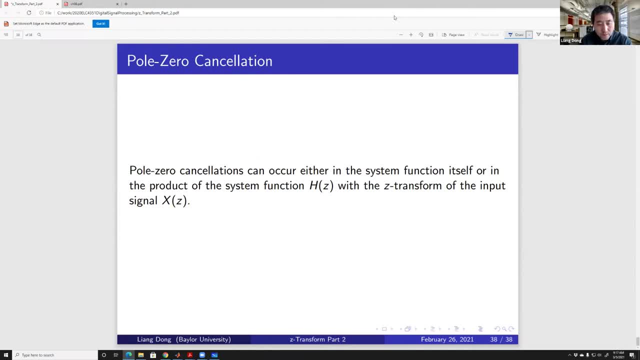 For this chapter is called as post-zero cancellation. post-zero cancellation can occur either in the system function itself or in the product of system function HZ with Z transform of the input signal X. So last time we kind of look at the output HZ times XZ. last time we are using an example. 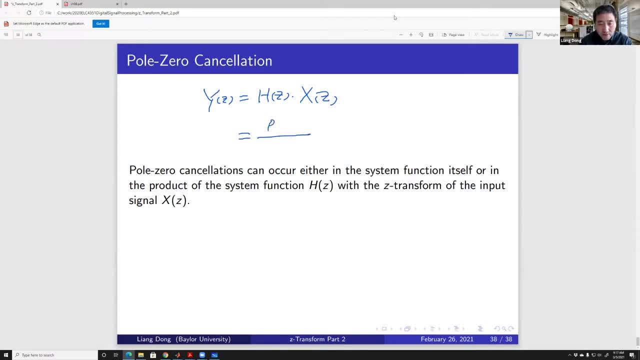 say. well, the system is linear time invariant. Therefore I have this rational form, BZ over HZ, And this input can also be put in two parts, numeric part, NZ over QZ, polynomial. So I have post here of my system, post here of my signal. I got zero of my system, zero. 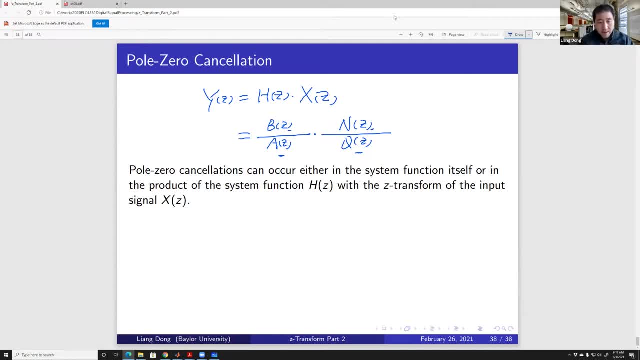 of my signal. So if let's imagine, if I have a pole of AC are exactly same as the zero which is the root of NZ, And those two can Cancel out. So this is a zero pole cancellation. Now the benefit of this is not so obvious in this, in this form. but let's say, if I 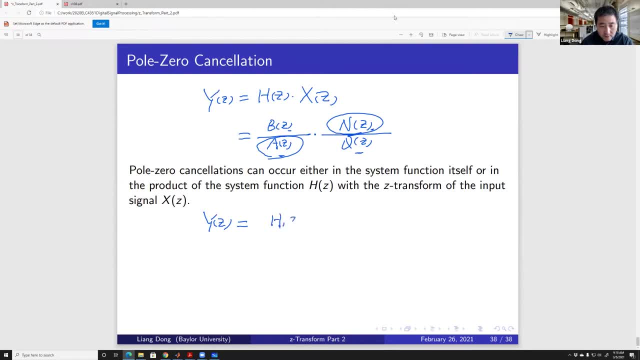 have a system called H1Z and then I deliberately cascade another system, H2Z, and then work on HZ. So if F1Z- the original system, is not stable, How do you tell? Well, I got a pole outside unit circle. 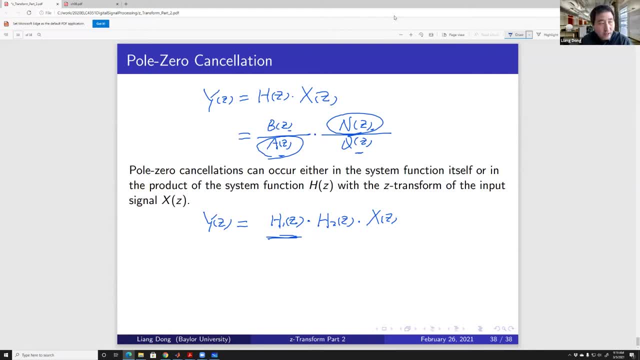 Suppose everything is called on now. suppose everything is called on now So I'm I can talking about within the unit circle, outside unit circle. So for color system to be stable the post should be within the unit circle. but I got. 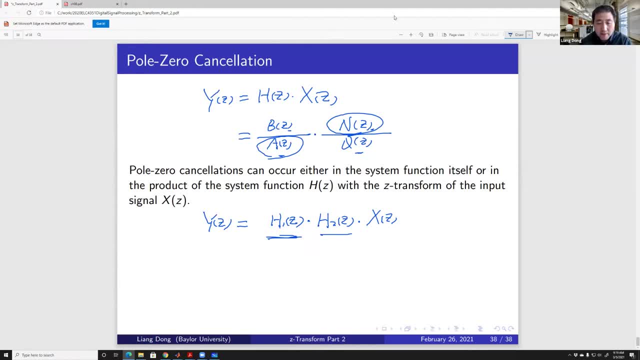 post outside unit circle. What can I do? Well, I can cascade another system, H2 that has a zero exactly at that position. Therefore, the zero will cancel out that pole And in the block diagram you have: Okay, Okay. 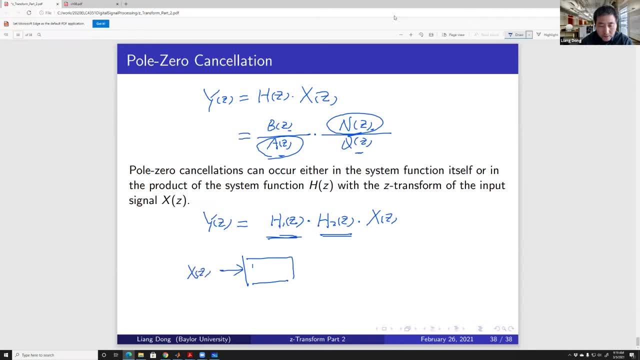 So what I do is I cascade another system, H2Z. It's designed such that the zero here is the same as the pole here, the, the, the, the out of bound pole, out of unit circle pole, And then we can cancel that and give us a very, very nice and stable system. 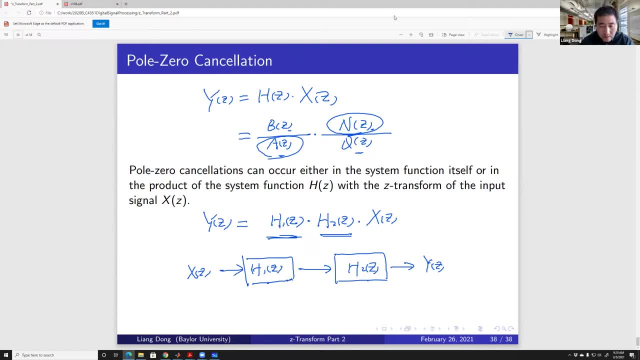 We can do this very easily. Okay, So system: linear time invariant system. it is. it is linear, So I can cascade, no problem, I can cascade, I can swamp the order, I can put in the middle of two system. 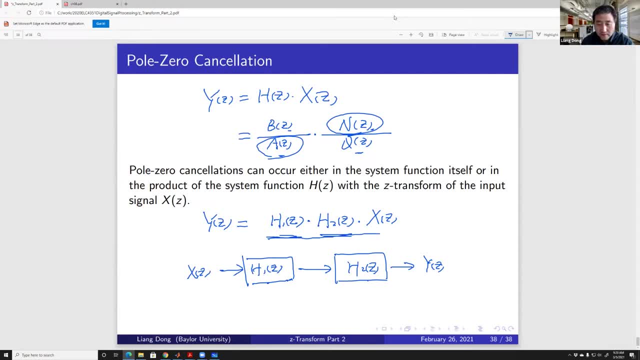 I can always do that, And in the Z domain that's product, So product. you can change this order, You can. I can plug another one in here. H3Z as designed, It doesn't matter. So it's really linear system. 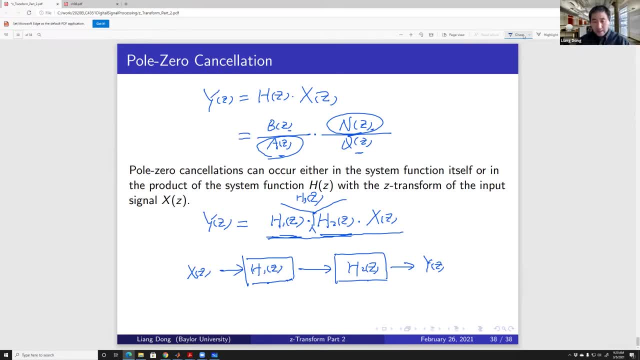 It's, it's a product in Z domain, I can plug those in And again, it's linear. So it's, it's really linear, Okay, So in any, in any case, it's, it's a very, very nice system. 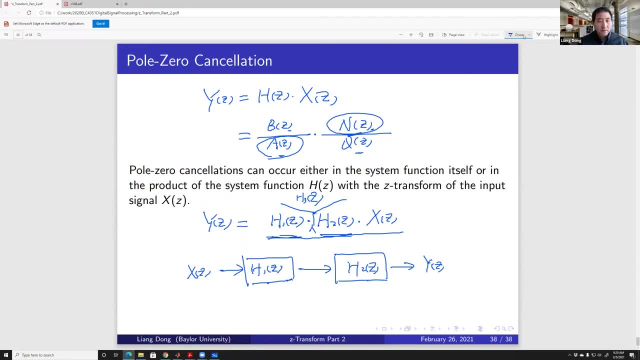 Okay, So now it's a real good system. We can make some problems, I can. I can make a problem, We can solve problems. Let me give you an example of a problem here. Okay, This is what's going on. 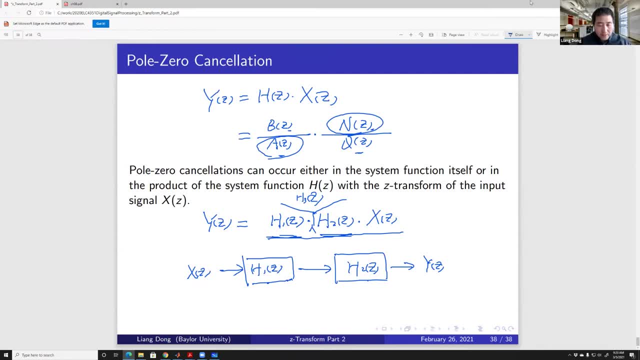 So let me do the Z transform over inz transform. So this is an example of a problem here. this is a, this is a company that's also doing something. Okay, They have this problem, problem of OK. So you see the problem. 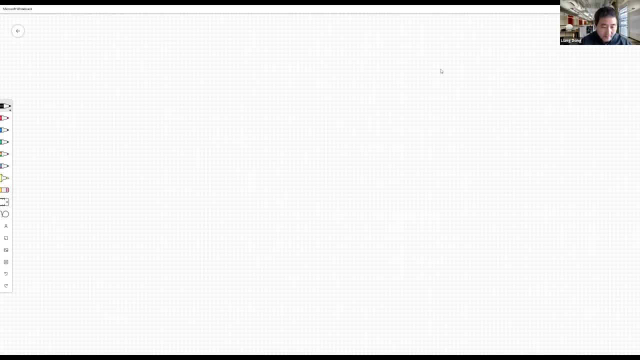 OK, You see this problem right. So this problem is getting stopped. So you see the problem is getting stopped. So you see the problem here of this, of the problem here doing a z transform, inverse z transform, in particular using the partial fraction expansion. let's say, this example is: i have a 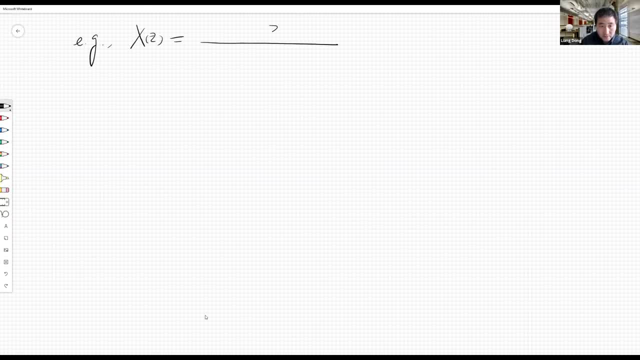 system or signal is written in this form. it's a rational format for z to the plus one. i want to find the inverse z transform. i want to find inverse z transform now. first, as we said, we always want to make this system function, or this function x of z. 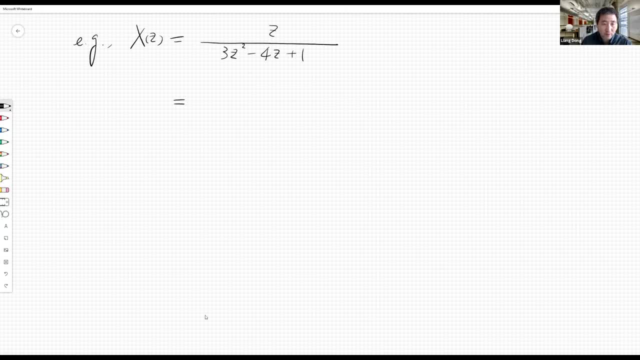 as a function of z, inverse of z z to the power negative one. it's just easy for me to to to do this inverse z transform. so we divide both numerate denominator by z squared. so we divide both numerate denominator by z squared. so this is second order. right denominator is two signal, so by z squared, so the numerate becomes z. 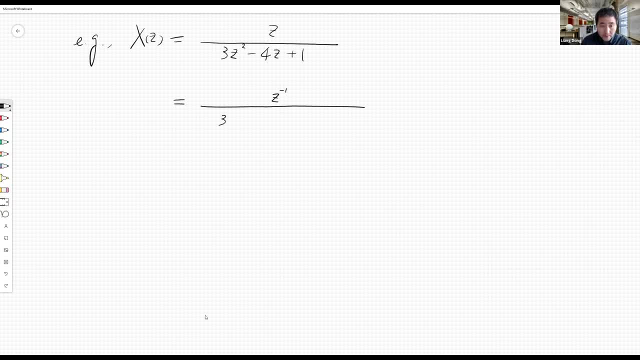 to the power negative. one denominator is three, subtract four: c to the power negative. one plus c to the power negative, two. okay, and then conventionally we want to make this: a is zero, which is the coefficient here, one. so that's subtract four over three c to the power negative. one plus one over three c to the power. 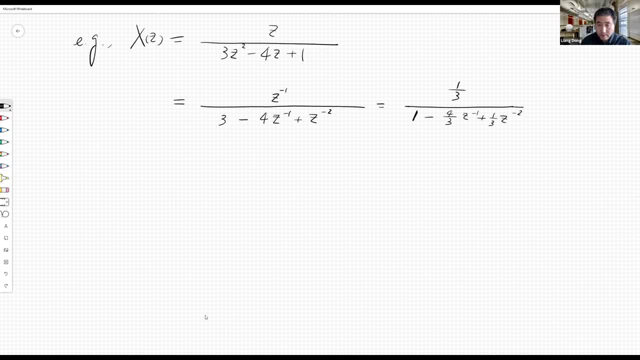 negative two and then the numerator is one over three c to the power negative two. why do we do that? one is usually this is indicated as h z, so if it's h z, you need to multiply this to the left of your equation and this term corresponding to y in current output. so i just want to make sure it's. 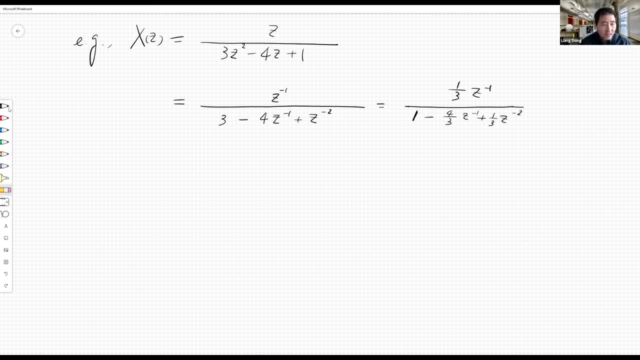 normalized. i pick up current output y in. so let's do a partial fraction expansion. now for this denominator. it's very to observe how to factorize that. so we have that one subtract c to the power, negative one times one, subtract one over three c to the power. one factorize the denominator. 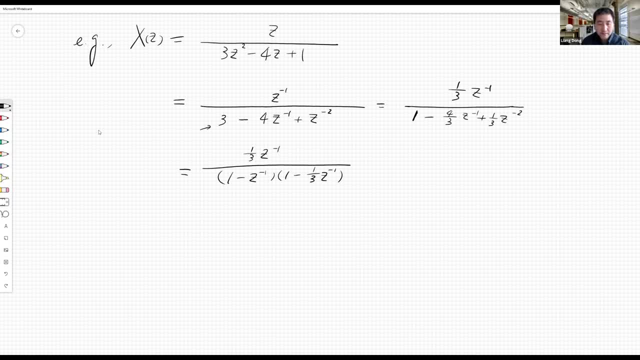 it may be easy from from from this format, but either way it's easy because the second order, i can do this factorization, and then i can write it into two parts. let me call this residual r1. one subtract z to the power, one plus. you see you, r2. 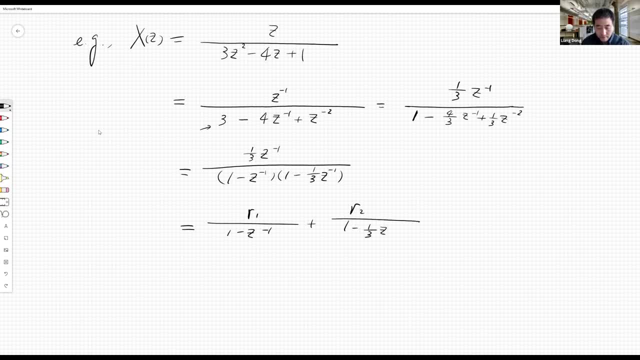 one. subtract one over three c to the power negative one. okay, so i got two post one and the one over three. i put that in two parts. i want to find the residual r1, r2. those are the aunts. so that's the one negative, r and r2. i want to find the residual R1, r2. those are the anyone. 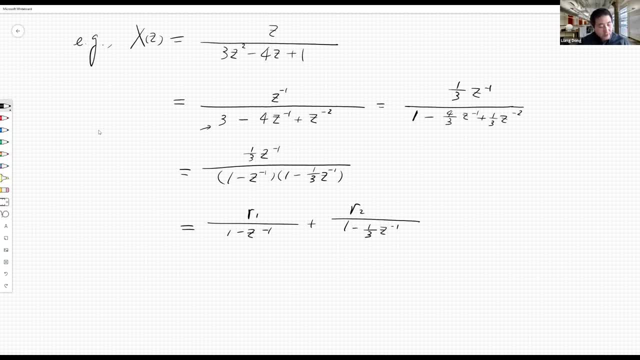 so there are three of you. okay, i also. i can put to a part one, one over three, i put two parts. so the Cay Almightye, the counterpoint of negative R1, always agrees with benerato to zero. so let's take this paint for this right here and then subscribe, and then from the left I can write: you see our. 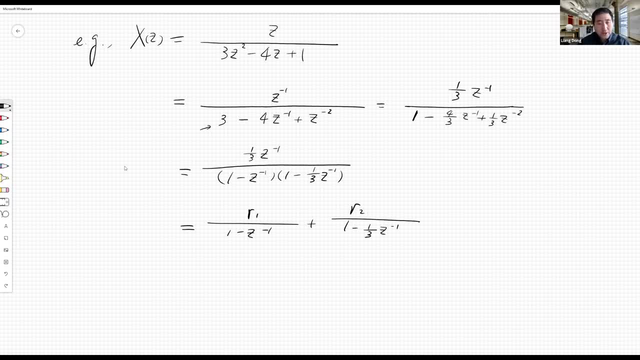 and R2, those are two constant- You can use the formula that we used in class. If we are dealing with a little complicated format- we will see another time some other examples, But in this case, because I only have two, unknowns. 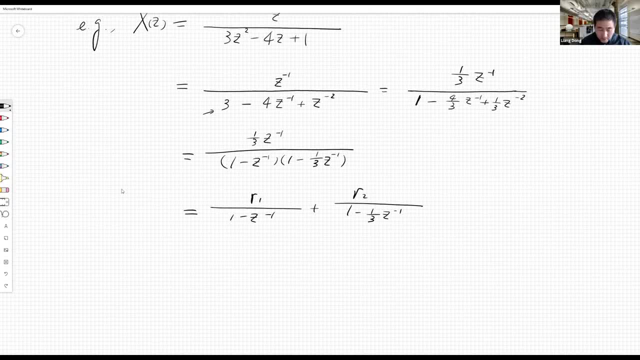 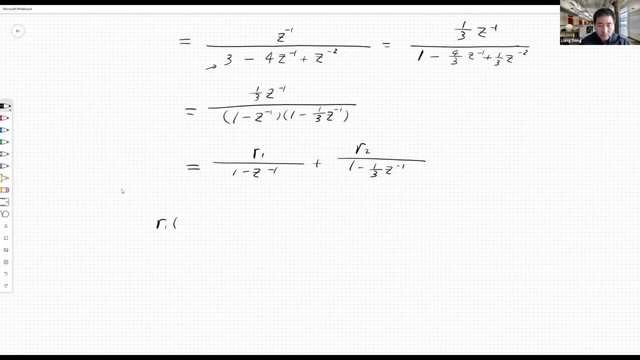 R1 and R2,. it's relatively easy to calculate What I do. I just, you know, multiply this and then make this R1 times. well, let me write out this: plus R2 times one, subtract Z to the power, negative one. 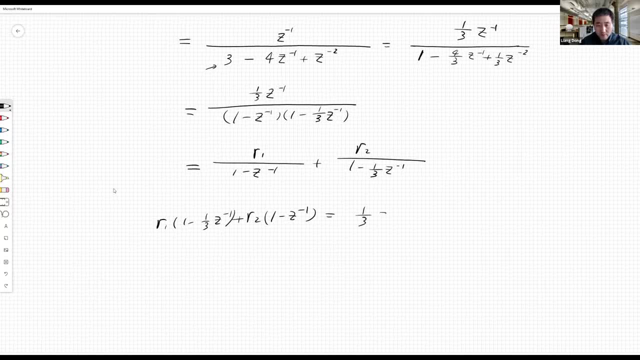 You know this is the numerator that should be equal to this. Therefore, I can write out this: equations for R1 to R1 plus R2 should be equal to what should be equal to zero right, And then negative one over three R1. 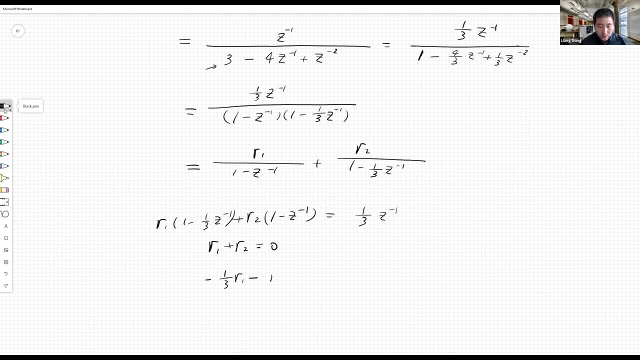 which is here Subtract R2 equals to that, equals to this coefficient right here, one over three, That's the first order coefficient. So in this case it's easy to calculate. So I'm just writing this to find R1, R2.. 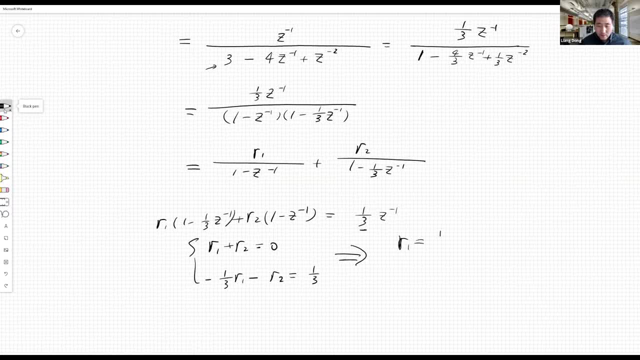 And then we find out, solving this equation. find out: R1 is one over two, R2 is negative, one over two. Okay, so for solving those two residues, R1, R2.. Therefore, my original function, the function of Z, can be written in this format: 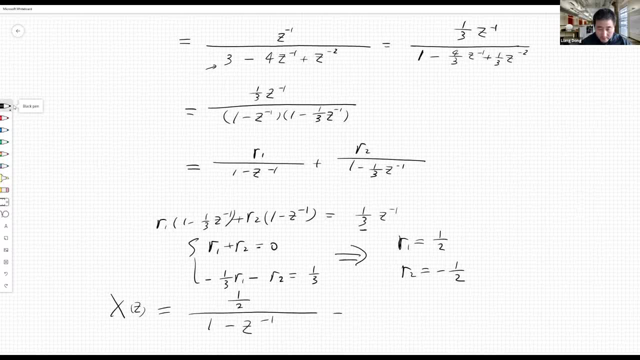 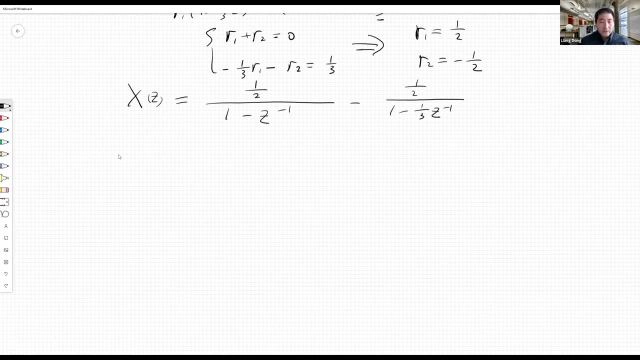 So one subtract Z to the power negative one subtract one over two, one subtract one over three, Z to the power negative, one. All right, so we got that. This is the final. this is the final for the partial fraction expansion. 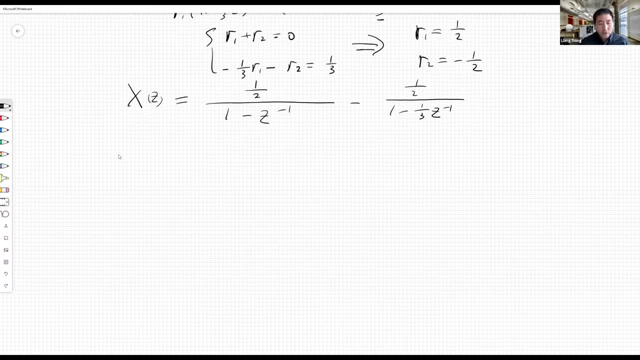 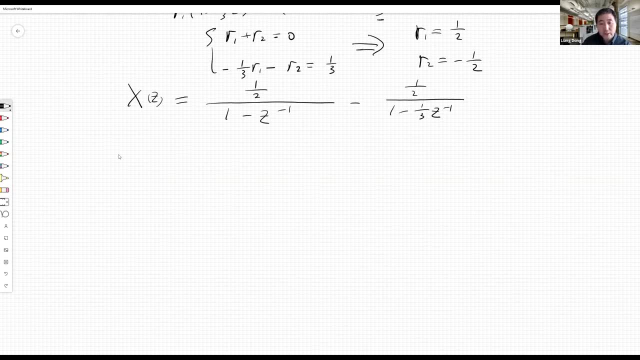 Now I need to transfer the inverse Z transfer back to the time domain. Now, remember, we are lacking the definition of region of convergence. I'm not given the region of convergence, So there are multiple answers for that. We know that I got two poles. P1 is equal to one right. 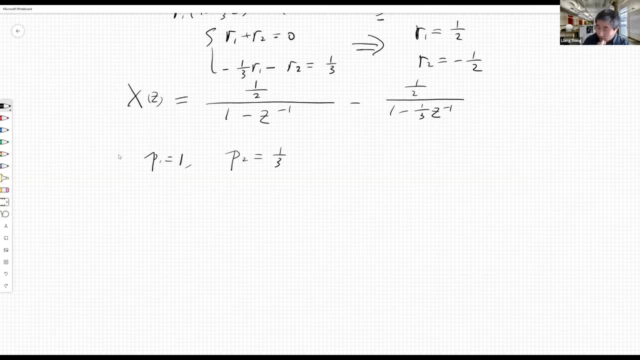 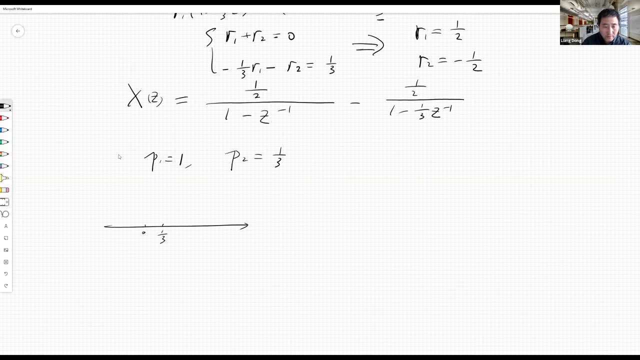 P2 is equal to one over three. It's given by those two denominators Similarly, as we had before. so we got a one over three here. It's a one here. I got a pole here. a pole here. Need to discuss about this situation. 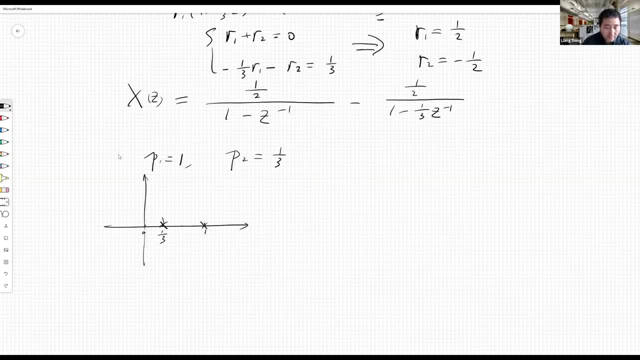 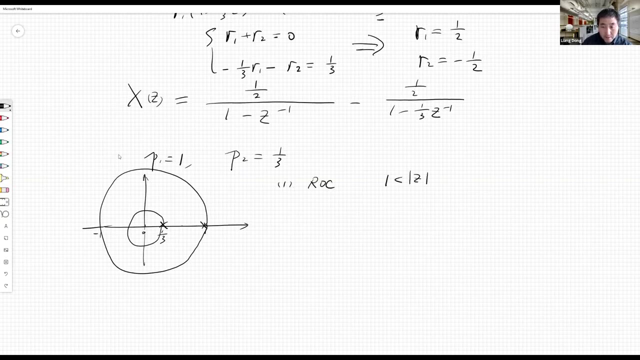 So we have- this is complex- Z plane. I have those two. It's not symmetric, but this is negative one here. So for the first case, if my region of convergence is is beyond the largest circle, which is one, So the first case. 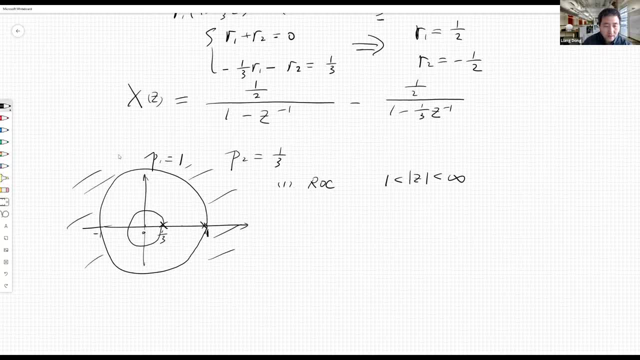 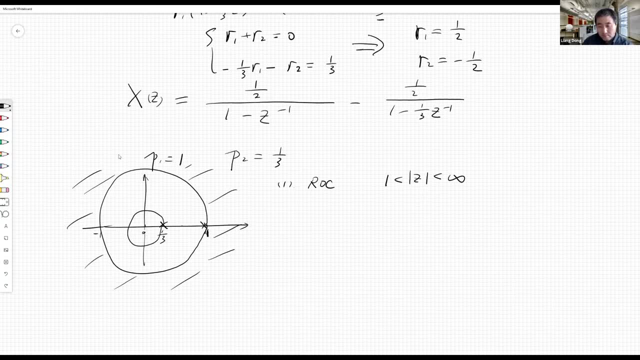 So the first case, regional convergence, is the external of everything, of those two poles, So it's from strictly greater than one and all the way to infinity. In this case, Xn, X1n. I call it X1n, equal to, it's a color system. 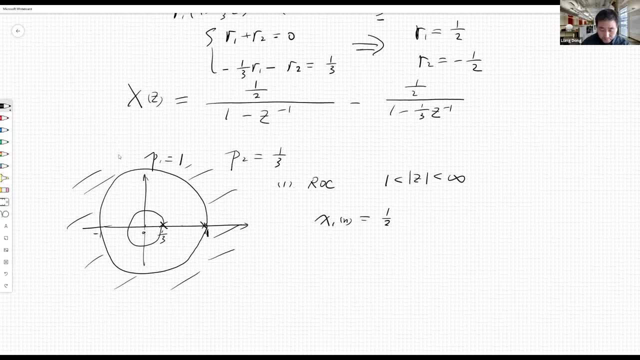 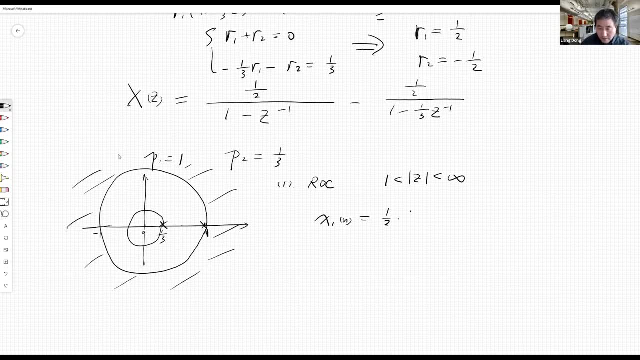 It's a color signal, So it's a half. this is R1 here. times: well, the base is one, base is one, one to the power n, So I don't need to write this out And then I write this: step function un here subtract one over two, that is R2 here. 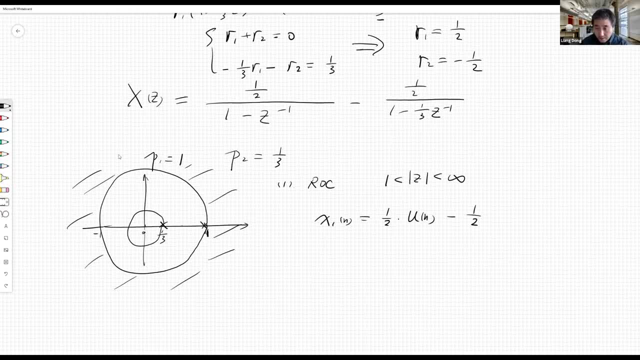 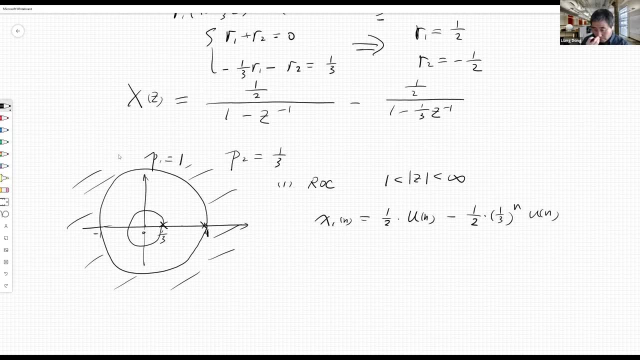 That's the second residual, And the pole is one over three, that's to the power n, And again, that's a quarter function. So we have that, And then of course I have some other possibilities: region of convergence, if. region of convergence. 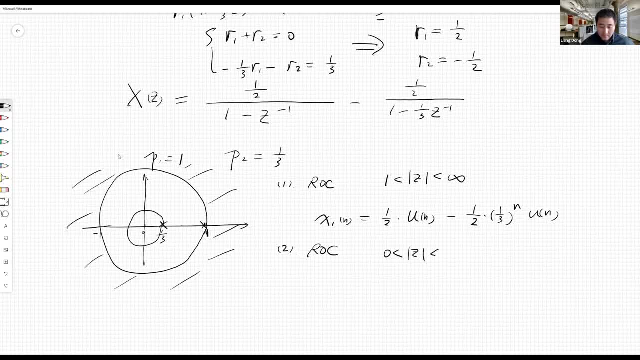 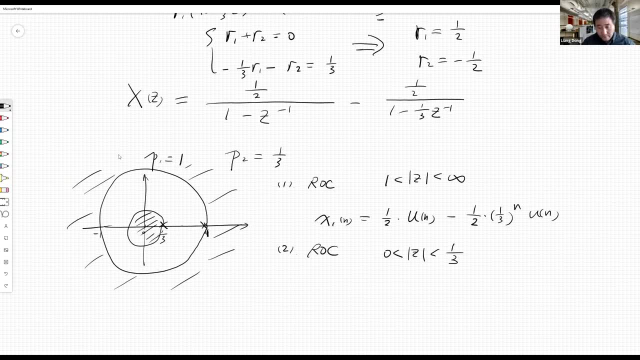 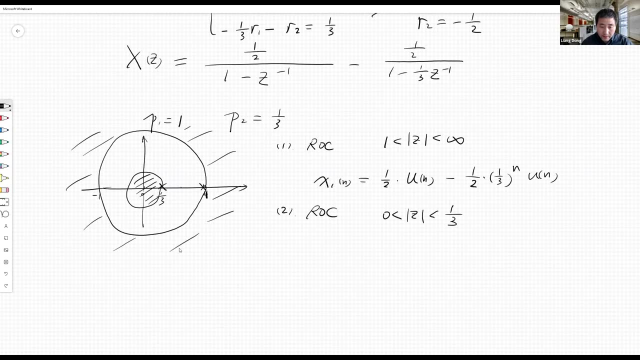 is in here. Less than one over three is in this region. in this region, then what I will have is I got my X2n. equals to half the first part. this is the second part: anti-causal, negative. 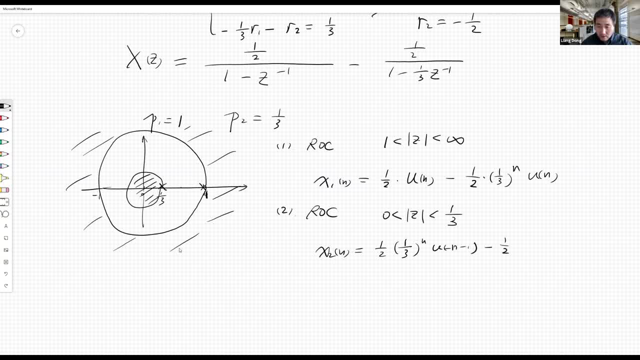 n minus one And the first part Okay, And the second part is also put a negative sign here. it's also anti-causal. so U negative, n negative one, Okay. So the entire thing is within. this is region of convergence, so within circles, and then 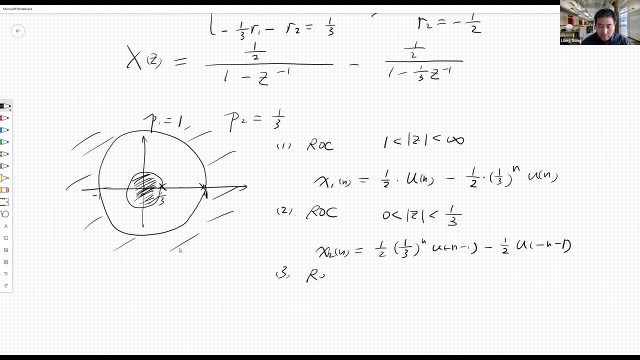 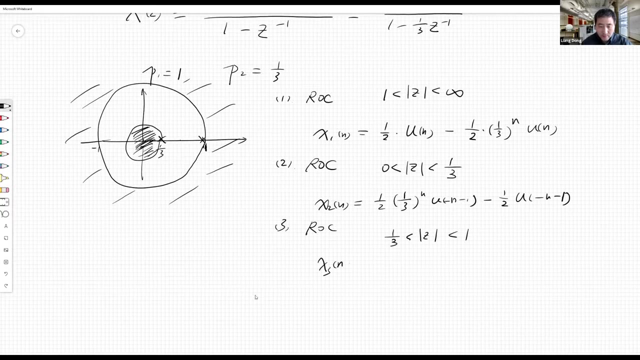 I have an anti-causal system. The third case is: region of convergence is in between these two, So in between these two radius, one over three, between one over three and a one, And therefore we can quickly write out this. the answer is this is the first part is anti-causal. 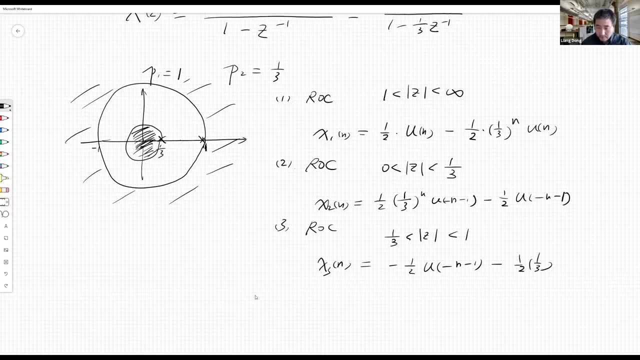 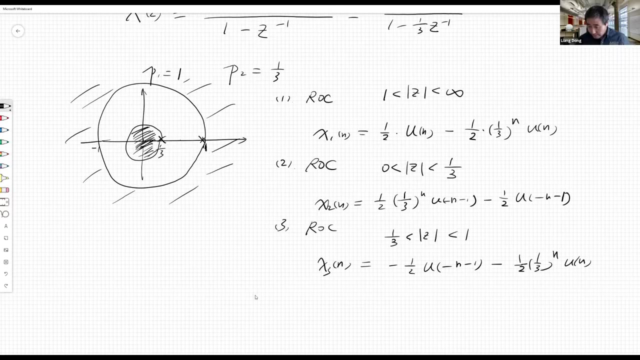 part And the second part is a causal part. The entire signal is anti-causal of U. Okay, So I have the answer for that. Those are the three possibilities- is depending on three different region of convergence. Okay, So let me use- let me use MATLAB example to check the answer. 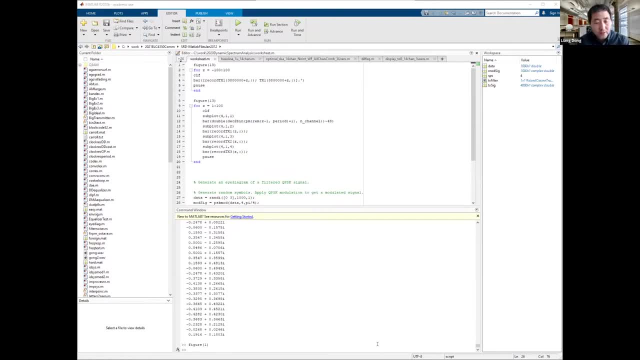 What I want to do is I want to use MATLAB to check with C, C transform, showing the C plane zero and a zero and a pulse, And then also showing a spectrum, showing on the unit circle what's what's going to. 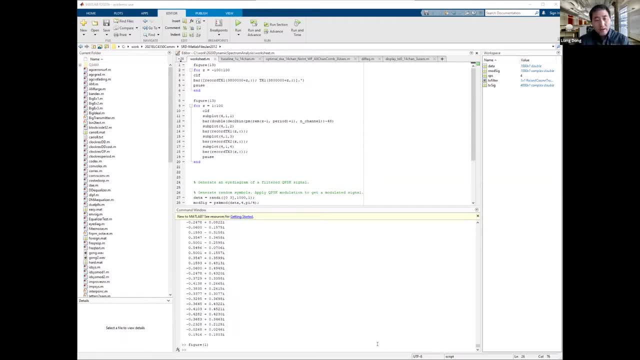 see what we're going to see in the frequency domain, Just get all familiar with some of MATLAB code. And again, for all this MATLAB code, The the program is, is very extensive and software is evolving all the time. I'm not asking you to to understand or to memorize every single command line, but you. 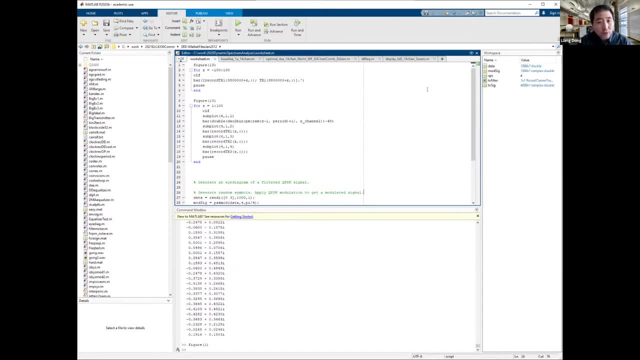 need to, I need to train. you have this ability, So you know some tool you can use and and a lot of those functions I don't even know. So I have to check what is the MATLAB functions, that the current functions for C transform. 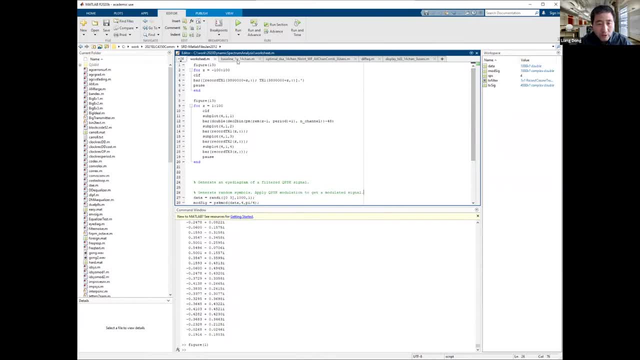 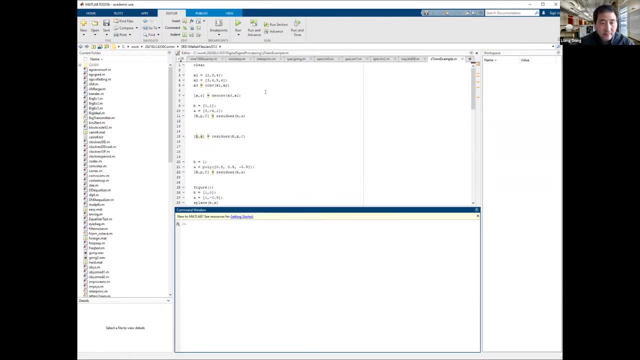 Now, with my knowledge, basic knowledge, knowing the theory of C, transform, I can, Using, Using some of the tools, very, very easily. I have a, I put a signal: X one, X two, and then first I do a convolution. 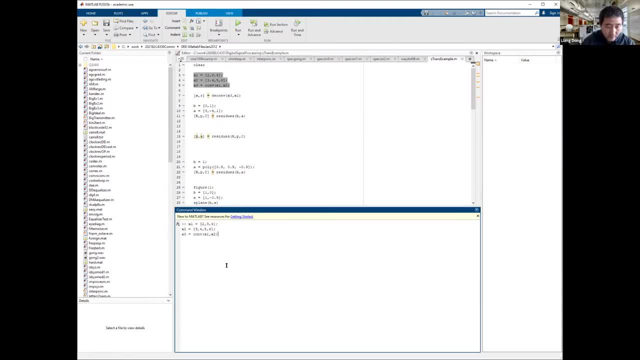 So here let me just copy that putting. So this is a, this is in the time domain. I'm doing a filtering. It's convolution. So I have two, three, four. convo was three, four, five, six. co-convo of X one. 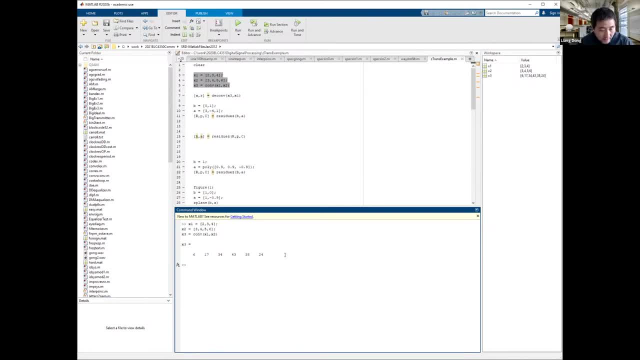 X two. I got this result And the length of this is the length of X one plus the length of X two subtract one. So in this case the length of the convolution result is six. There is a command in MATLAB. actually we can do deconvolution. 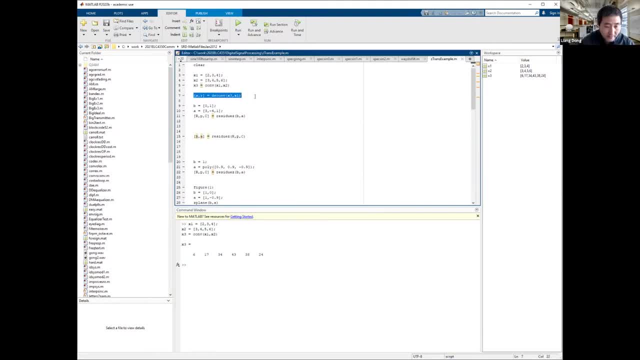 So deconvolution is written here. Let me copy this line here. So deconvolution is I'm- in this case I'm deconvolve- X one out of X three. So it's almost like we are doing a long division, a polynomial division. 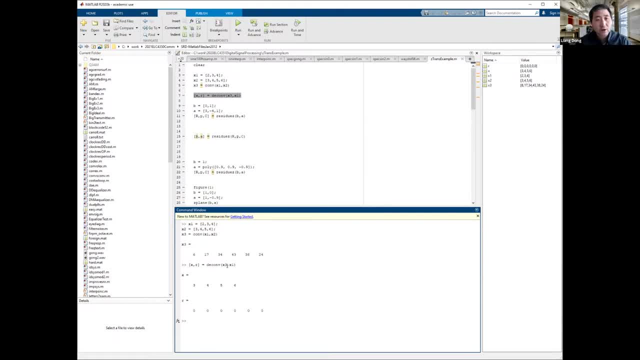 If you think that X three is a factor, those are the coefficients of a polynomial. X one, Those are the coefficients of a polynomial. So we are doing a long division of two polynomials. in that case X will be the quotient and R is the residual. 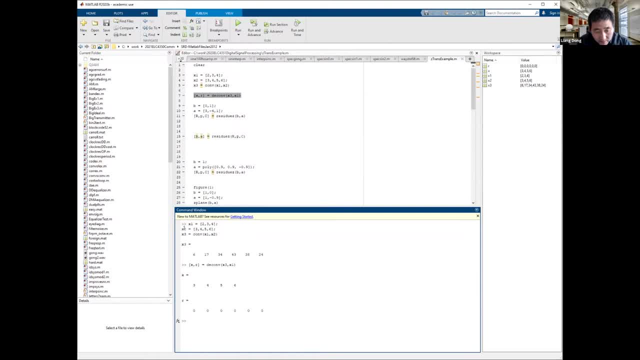 So in this case we are X. is this X two, three, four, five, six, exact eyes or zeros? I don't have that. That's all zeros. So the residual is zero, because I can do this long division perfectly. It's coming from X one combo with X two. 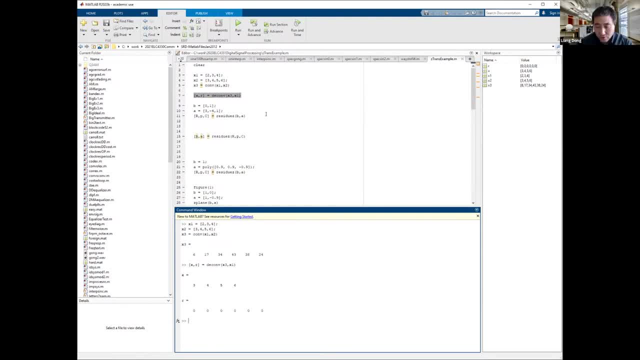 So we we can easily show that. I'm just showing you before I'm getting to Z transform some of the common code. I understand that you can check your answers using deconvolution as well. Okay, So let's see. now for the problem. I just have write out this again. 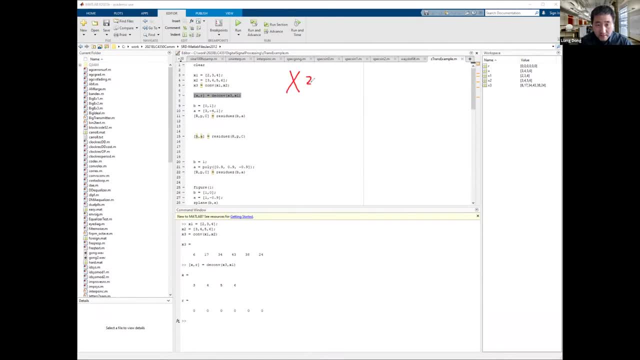 The problem I had is a problem I have- is X Z equals two C over three C square, subtract four Z plus one right. This is the problem we just worked on. So if you look at this format, the polynomial, The numerator, in this case the coefficient are zero and a one. zero and a one. 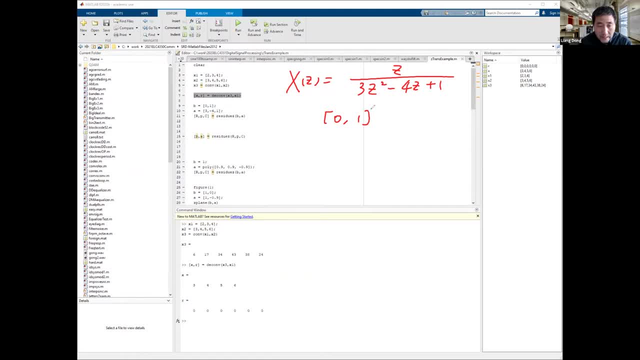 And the polynomial one is because I have a one here And then the polynomial of denominator is three native four and a one You may have, you may. it's not, maybe not that clear here, but if I am putting everything. so if I change that, the second is changed. 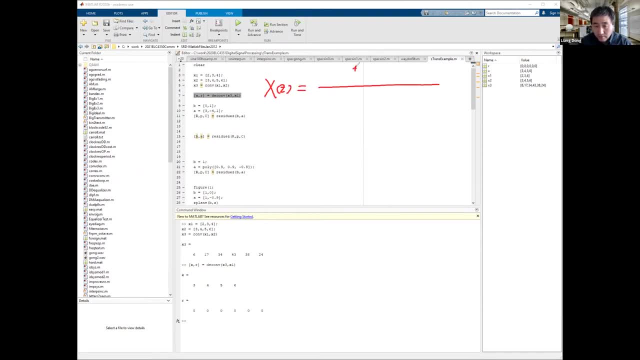 It's changing that as a function of a Z to the power negative one, you divide C to the power two on both numerate and denominator. So this is what I have: three subtract four, C to the point of one plus C to the point of two right. 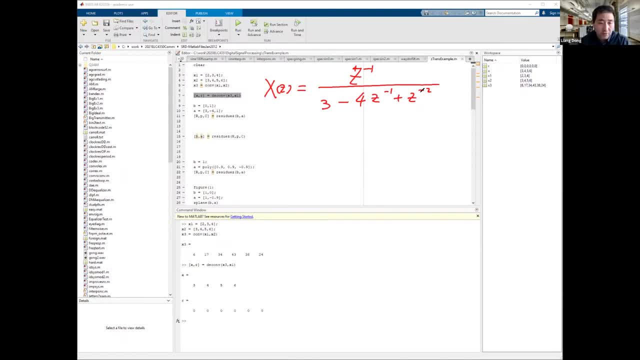 This is what we have commercially. We got this format and then it's easy to understand that B is a function, B is a polynomial with coefficient zero and a one Zero is the coefficient B zero, which is of C to the power zero which we don't have. 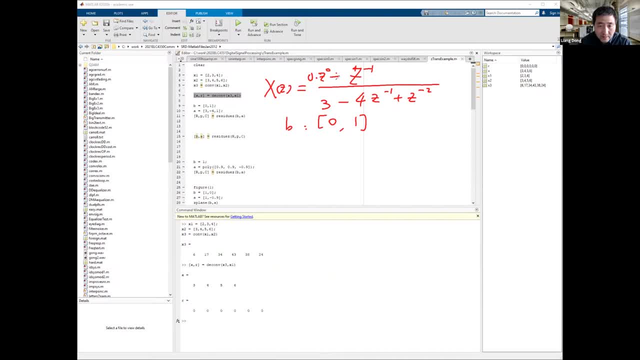 here, which we don't have this term. The second term is this one here. That's the key, Okay, And a in this case is three native four and a one is out here, right, So so we are using this to represent this system function exactly, or this function. 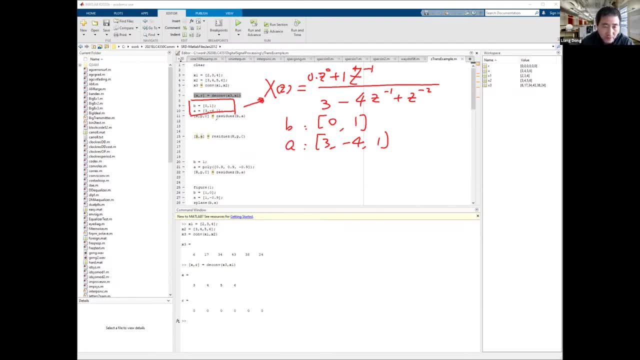 And then what we do is we are using A command called residual Z, B and a. that is going to give me- it will do- a long division, So what it will give me, it will give me, ah, which are the residuals. 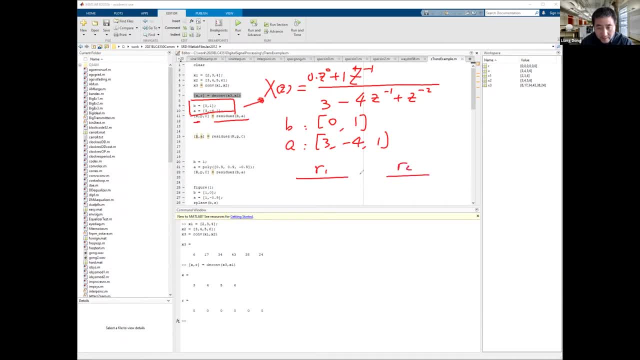 Those that are one or two. if you remember, I have in this problem. P is is a vector of post. So one subtract P one, one subtract P two. Okay, Those are good, Give me those P one, P two. 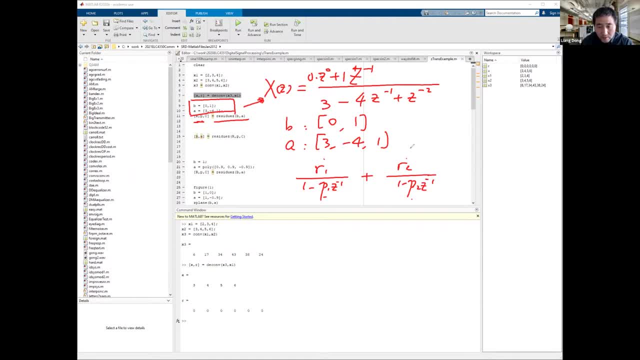 Those are in the vector of P and the R is the vector of this, or C, R one, R two. So it's kind of doing this partial fraction for you already, numerically give you the answer. And then C, C is, C is when you divide the polynomial, it's a quotient, it's a quotient. 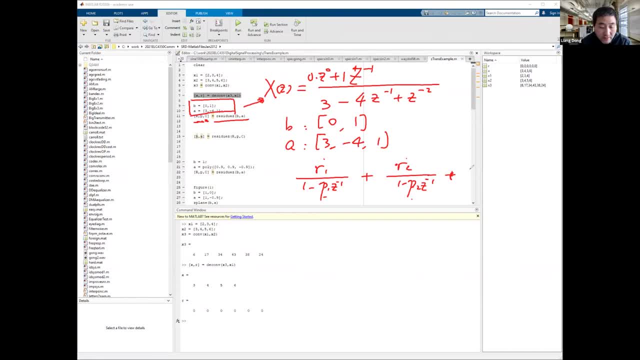 So in our case we don't have that term. Now, if this is improper rational format, I will guess I'll have something here. I'll have something here, Okay, But in my case I don't have that. It's all zero, because it's proper rational format at the very beginning. 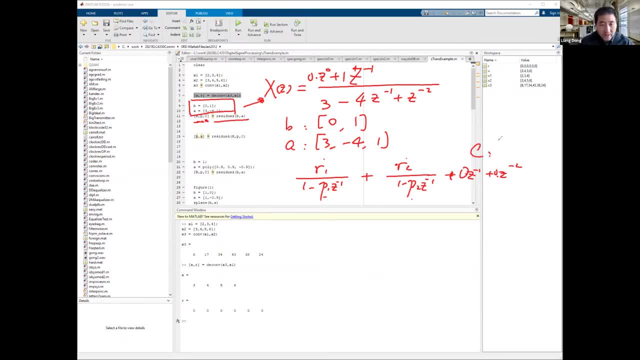 So in this case, C should be all zeros, Okay. So let me work this. I copy that. Okay, Now this is what I have, And I have: R is 0.5, negative 0.5.. That's exactly what we calculate by this: one over half and negative one over half a Poe. 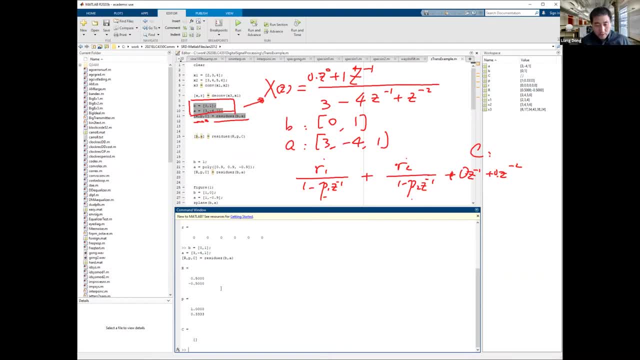 is one And the one over three. those are the two poles and a C. as we understand, the C is an empty set because I don't have the quotient part. So very nice, I think that's how it can check the partial fraction expansion for us doing a long division. 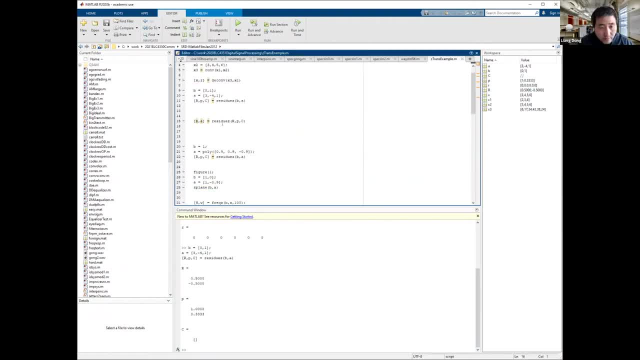 and give us all the audiences here. The residual C can work both ways. If you have all these- the residual, the Poe and the quotient part- And Using this, the same command, you can find out the coefficients B and ACE for the polynomial. 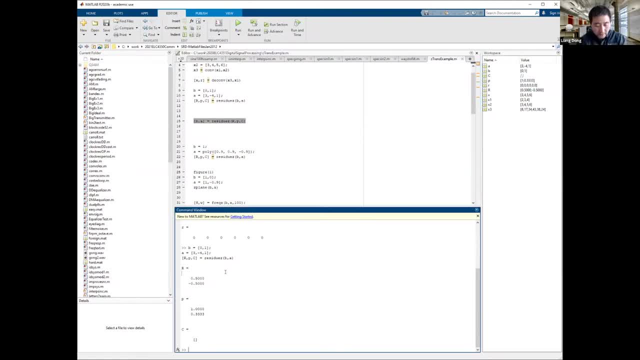 for the polynomials on numerator denominator for my function X. So let me do this so you can see I got I recovered back. B is the vector of those two coefficients, where the first one is zero, The second one is one over three. 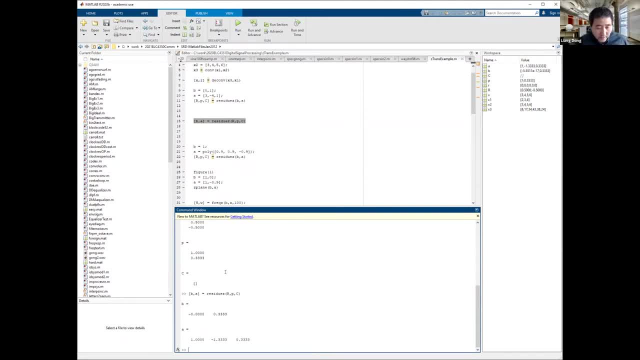 A is the coefficient of the denominator. It's one negative, four over three and one over three. Okay, In this case, because everything is normalized. this is everything is normalized. where you get, where you get, is you got this equal. to remember, we also calculated one over three. 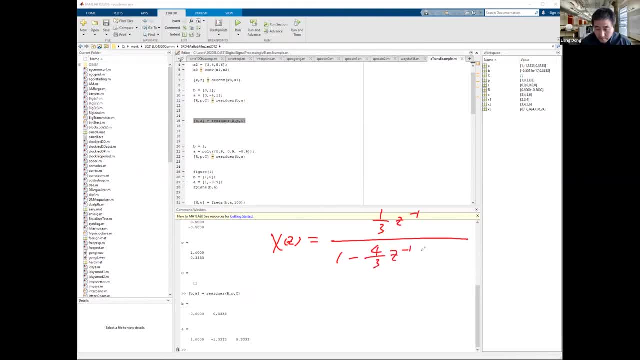 one subtract plus one over three. C negative two. you, you got the. so these are the coefficients. Let's see: A is coefficient here. B is the coefficient here. Okay, So very nice, We can always check. We can always check this answer. 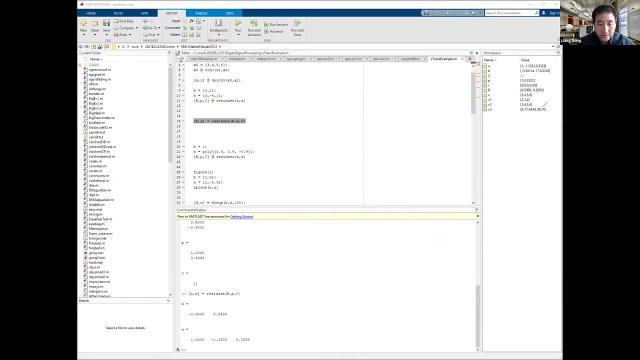 Even more in MATLAB. let me continue to show you here. So if I, if I only know the post, I do not know the polynomial coefficients, That's okay, Because in MATLAB you can. you can generate a polynomial given its roots. 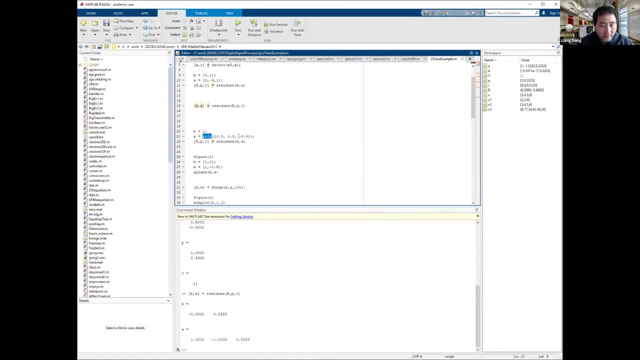 Generate a polynomial given its roots- Suppose I have roots- is 0.9, 0.9, negative 0.9.. So those are the roots for this polynomial and I'm putting as a coefficient for a. therefore, these are the three posts right. 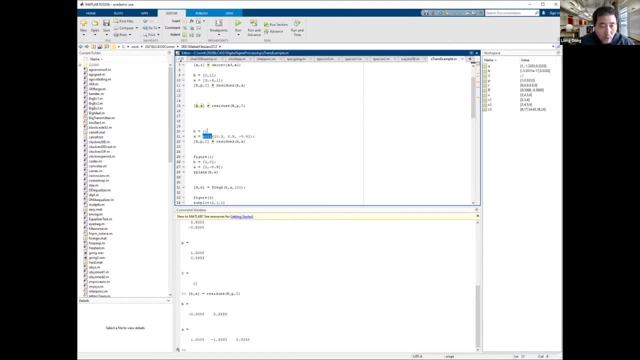 These are the three posts and the B is one. So, numerator, that's just one over that, And then I check with my answer at the same time. let me plot this out and do this So we can see. now I find out. 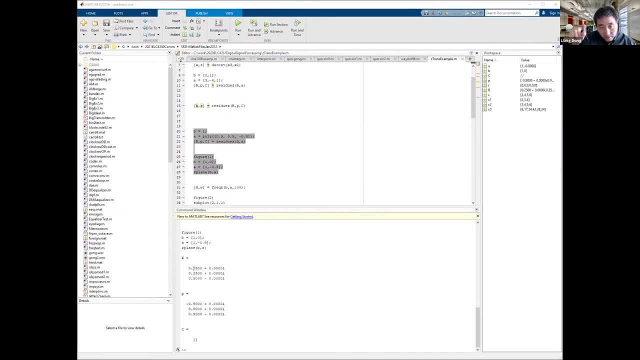 Okay, The R is the residual, So these are. on the numerator right It's 0.5, 0.5, negative 0.5 P. P are the three posts. should comes from this polynomial. should polynomial generate by those three posts or by three roots? 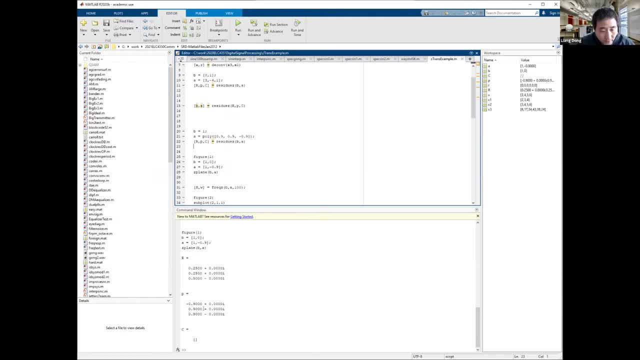 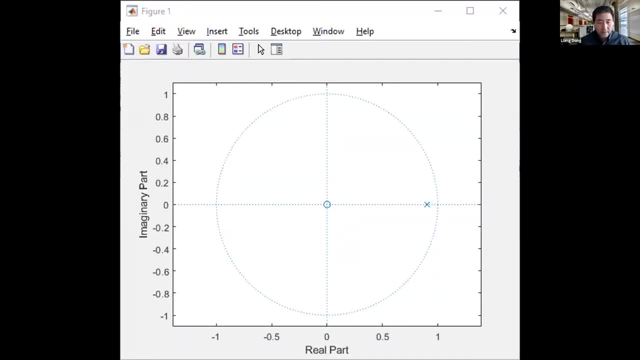 So the post should be exact: negative 0.9,, 0.9,, 0.9, and then the quotient part. I don't have that. That's what was empty. Okay, So this is when I type in C plane. 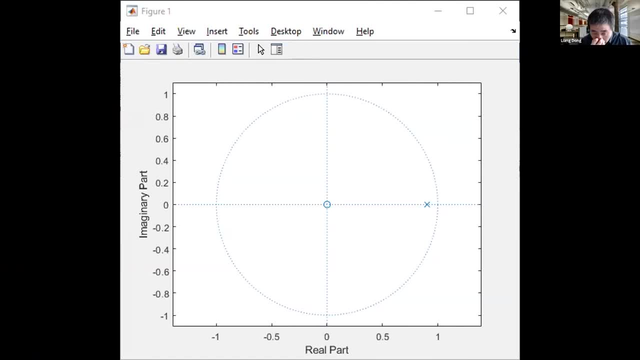 Okay, B, comma a, I give the coefficient of those two polynomials and it will show me something here. And in this case, in this case it's a. I'm particular, I'm just using a, a zero at origin and a pole at 0.9.. 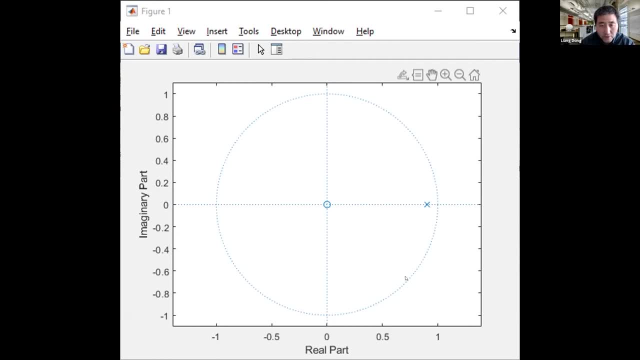 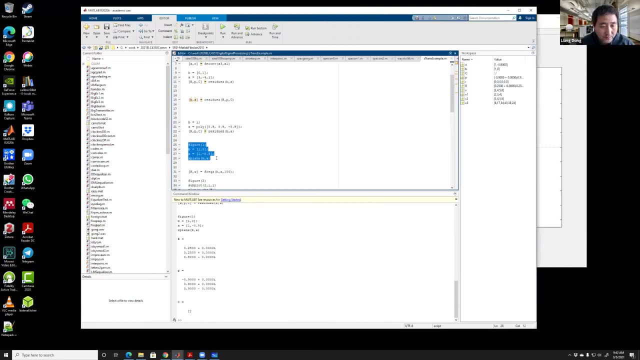 So you can plot this out very nicely, draw the unit circle for you. So it's here. Okay, So you can see what I did here. This, this is a figure of one I brought out. D is one or zero, actually just one. 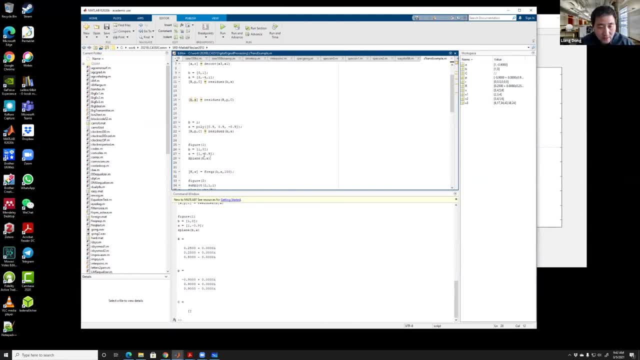 A is one and a native 0.9.. So what is that, Well, that will give us? that will give us one over one, subtract 0.9 C to the 0.8 of one. So this is what I have. 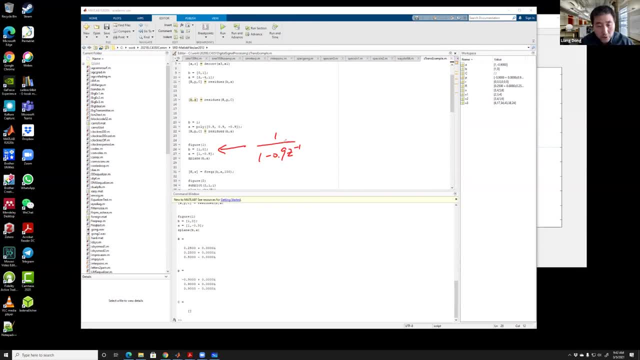 And I I have a zero of a zero at origin. I don't have a zero in this case, It's at the origin, usually omitted, And then I have a pole at 0.9.. Okay, So that's what we have here. 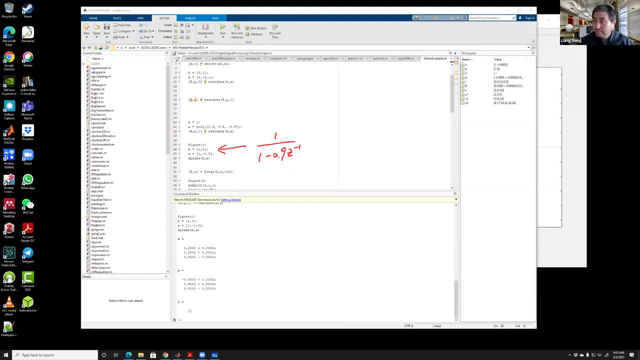 Exactly Okay, That's what we have here, So you can use a C plane. Very easy to show that. Now I also want to show what if I'm travel along the unit circle. as I explained, when I travel along the unit circle, I'm checking with the frequency. 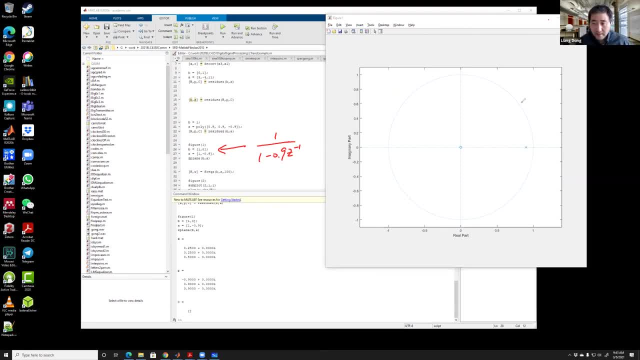 I mentioned this again again. later We will know that's exactly this: the the bridge- I will call this a bridge- between Z-transform and Fourier transform. So Z-transform is a general case, Fourier transform is a special case. I'm not going to check with all the Z values, I'm only going to check. 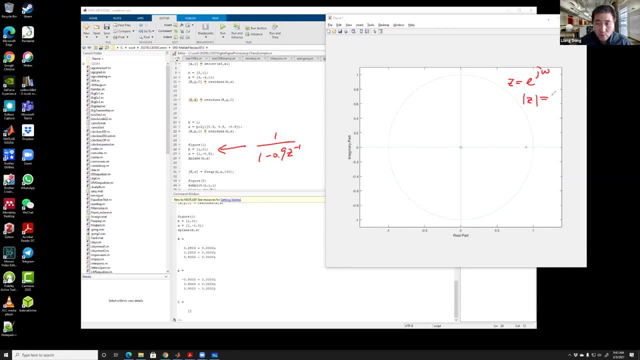 Z value when the mole of Z is one. So I'm only going to check on this unit circle and travel along this unit circle. That's where you get the special case of Z-transform, Fourier transform on the Fourier domain. So I also want to show the same B and A here Now I 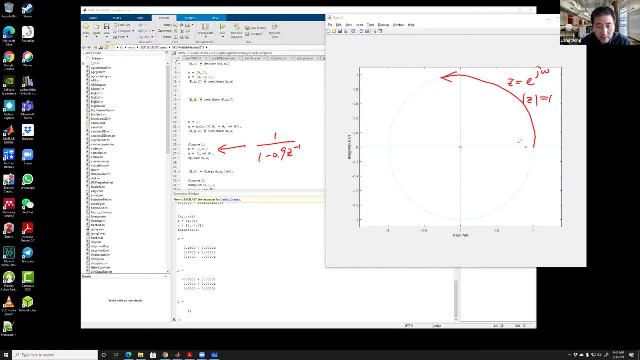 know it's zero here. a pole here. Let's see how it looks like in the frequency domain. Before I draw this out, I get a feeling I'm traveling along this unit circle. So if I'm here at this point, which is DC, my frequency is zero. right, This frequency here is zero. 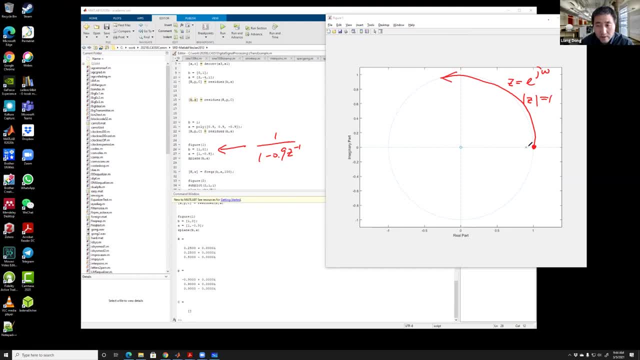 And it's close to the pole. When it's close to the pole, the value of XZ should be quite large, Because it's close to the pole. If you draw into the pole, then this value becomes infinity. Then I travel around. Zero is in the middle, so it doesn't affect too much, But I know. 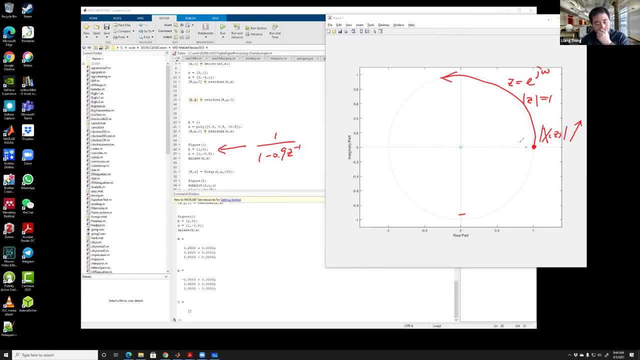 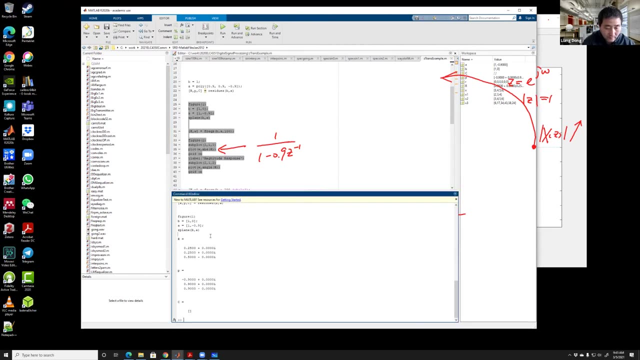 when I close to DC. I got a quite large response, So let's see here. Now I am doing both of the two part here, Hi. So On the second pot here, what I did is HZ is frequency. We showed this once before. frequencies is going to show me a spectrum. I also using polynomial 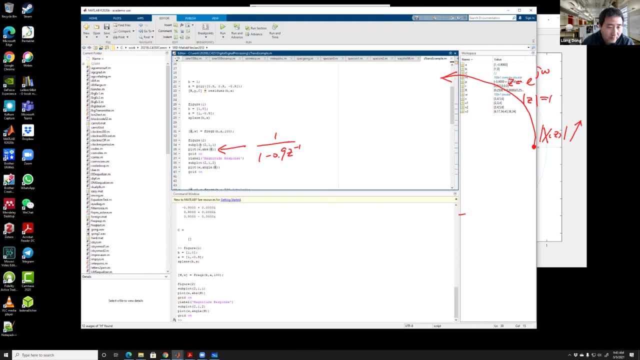 coefficients B and H is the value, W is the frequency, So I process, spin, W plots fringe. Okay, w an absolute value, h, so i plot. the top picture should give me the amplitude or the magnitude. the bottom picture is angle of h, so it gives me the face, face of my output. 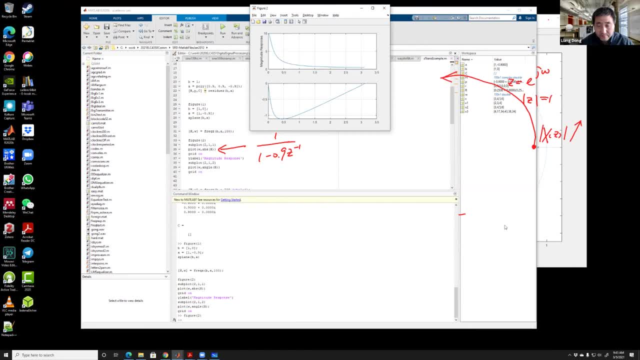 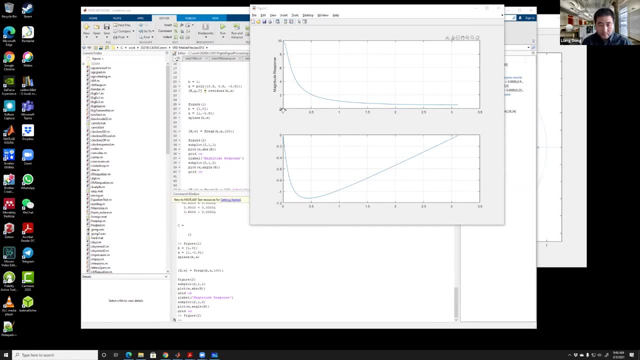 so let's look at here, that's what we have. so, indeed, i have something. this is the magnitude response at zero, because i'm i'm closing to the pole, so it gives me a large number as i'm going for further, further, it's just giving me a smaller. 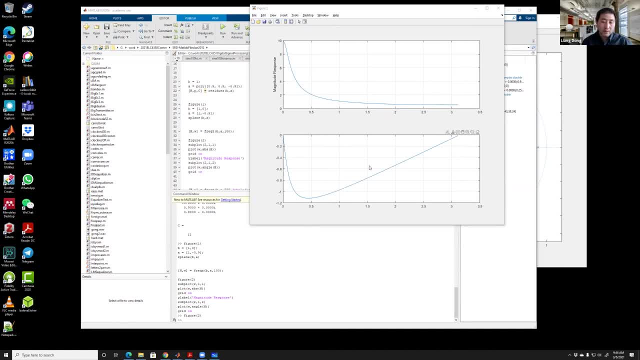 number and the the bottom picture showing me this face, but the face is non-linear. this is highly non-linear. why is that? well, because this is infinite impulse response. iir system. right, you got a feedback. you have something on the denominator. that's the feedback, so you will. 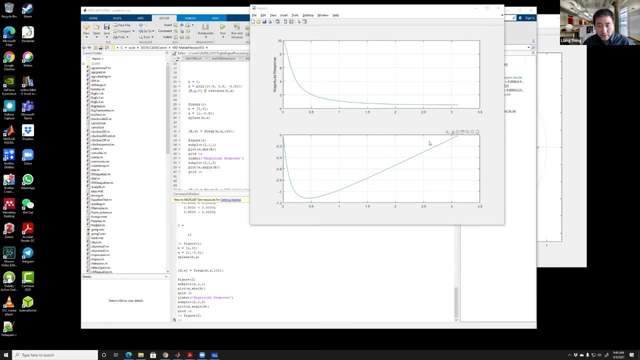 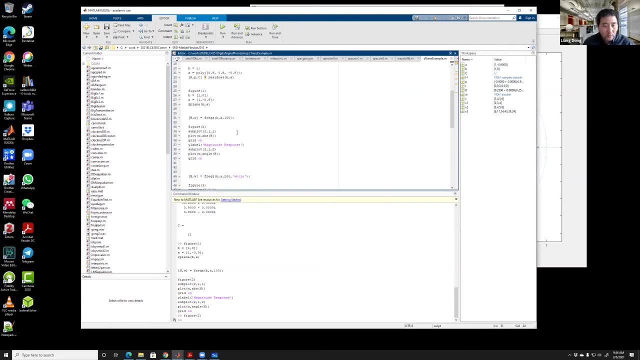 have a non-linear system and that showing in the face that's not a straight line, it's just some curve, okay. so let's try another one now, if i'm going to draw the frequency risk, the frequency spectrum of the entire from zero to two pi, and then what you can write is: you can. 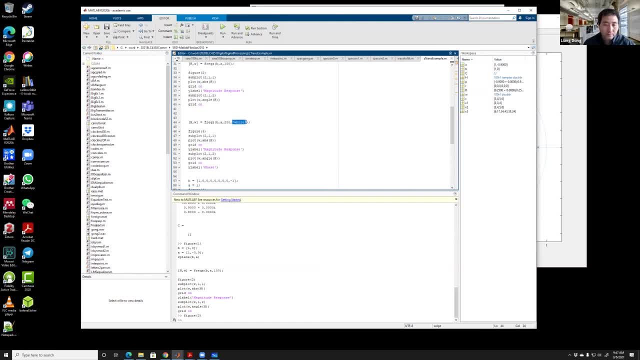 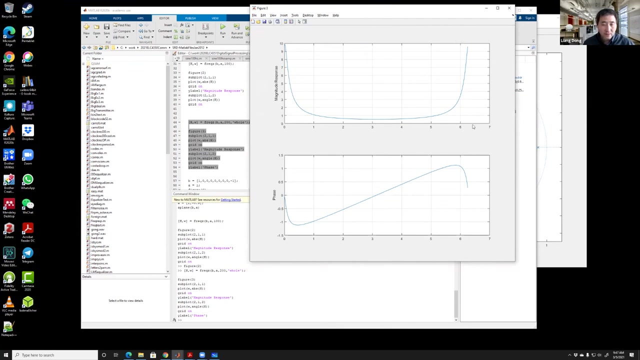 write that i want a whole, whole of the spectrum and i'm plotting out 200 points and i draw this. so let's see, and it's all the same here. but the only thing is i'm going to use, uh, 200 points. it's from, from zero to fs, to sampling frequency, or from zero to two pi, all right, but we know we don't. 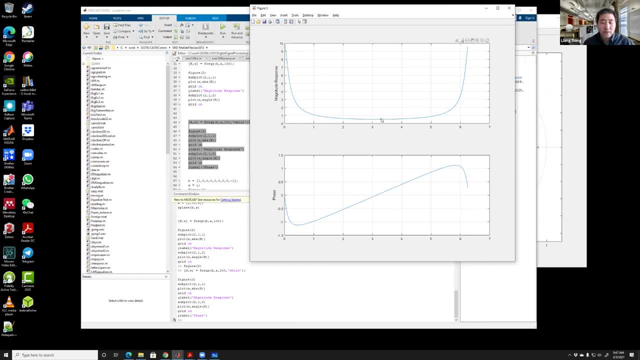 really need that, because beyond that crystal rate everything is a mirror image of itself. so you have the redundant information. that's why our original layer. we don't need a hole. we can just plot from zero to pi. that's good enough. in another word, when you travel along the unit circle, 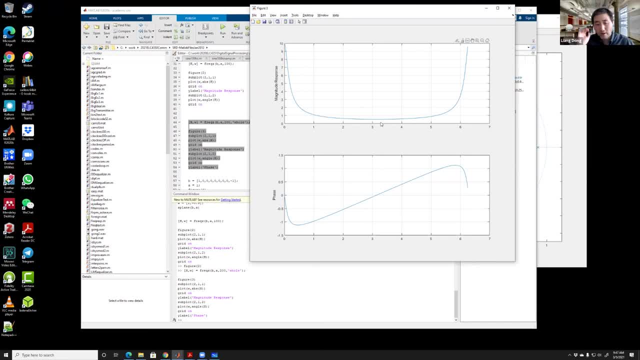 you just go half circle from zero to pi and you got all the information or everything that should be there. and then the same thing here for the face term on the bottom picture. the face is also. it's a mirror with the center at the pi or fs over two. 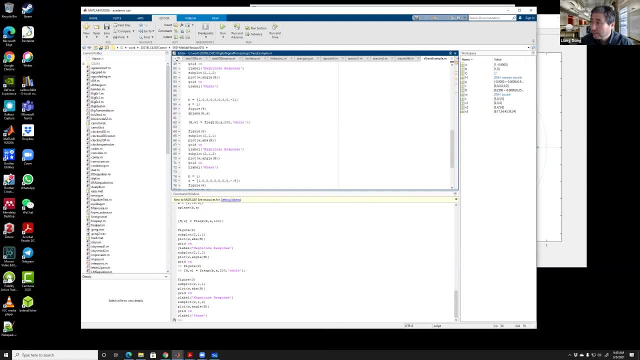 so now let's move to something that is that is interesting. let's see if i have a special, special case i designed here. all right, so this is my b and this is my a. so b is this vector. those are the coefficients. so what we have here is is: is: is one plus zero times c to the power, negative, one plus zero times c to 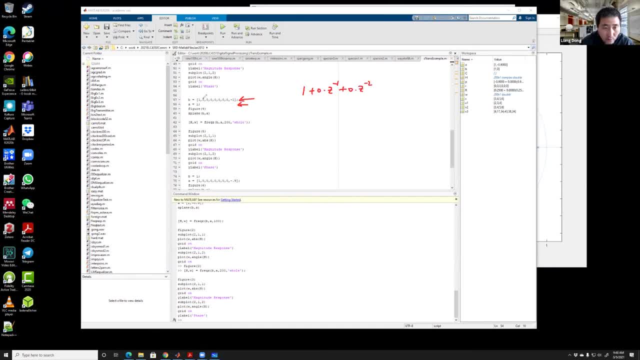 the power negative two. how many? we have one? this is one, two, three, four, five, six, seven, eight. so we got the last one is subtract, subtract z to the power negative eight. so i don't have the middle term, so the entire thing is one: subtract z to the power negative eight. on the numerator, and then the denominator is just one right. so 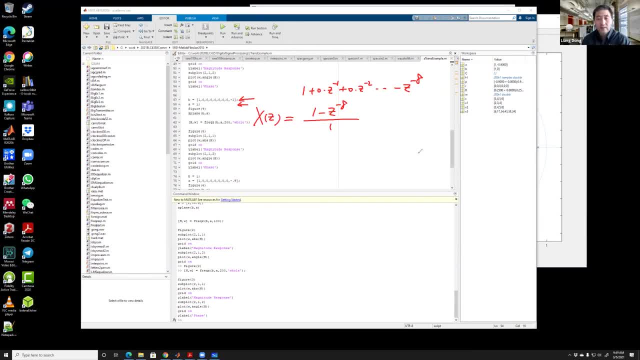 this. this is my signal in the z domain. we got that um. we process z plane within this coefficient bna. we don't have a pose, but implied those posts are at origin. it's going to show you, but we don't, we don't really count those. where are the zeros? well, zeroes need to make sure. 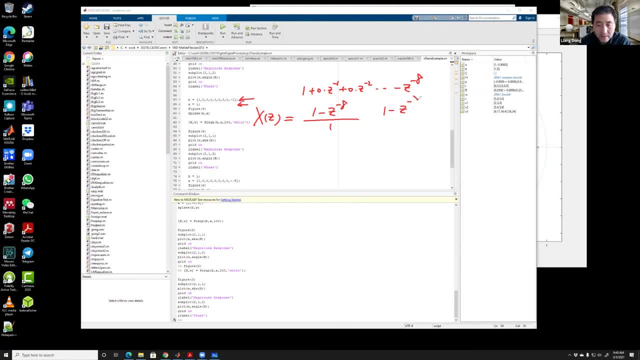 that the numerator one subtract z to the power negative, eight equal to zero, so z to the power, eight equal to one. and what are the solution for this equation? uh, so it can be positive, negative one or positive, negative one. right, z can be positive, negative, j. well, actually z it is. uh, if you draw this on. 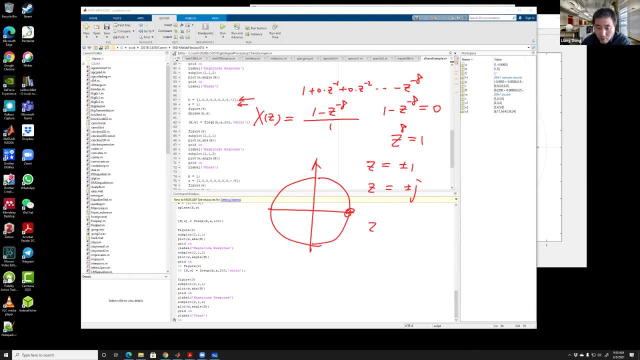 the unicircle z can be taken. this point, this point, that's positive, one, negative one. positive j, negative j z can also take at this point, this point, which is one plus j divided by square root of over two. so you can also be this, z can also be. 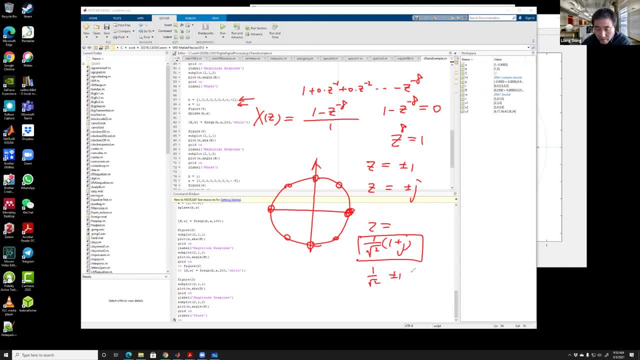 it's a positive, negative one, positive negative j. so those are the four points here. right, because z is a complex. we see the complex number. so, solving this equation, you are going to write out: this is equal to um, e, to the power j, two, two pi times k, where k is integer, and then you can. then you find out z is equal to: 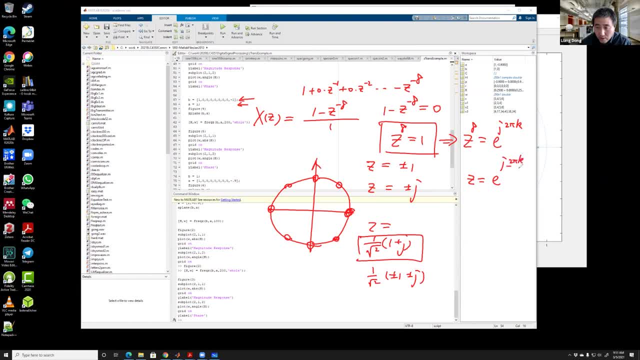 e to the j, two, pi, k over eight, where k is an integer. so in this case k is zero. one, two, three, all the way to seven, and then you beyond seven, you got eight, you got eight, and then you got seven, and then you got eight, and then you got seven. 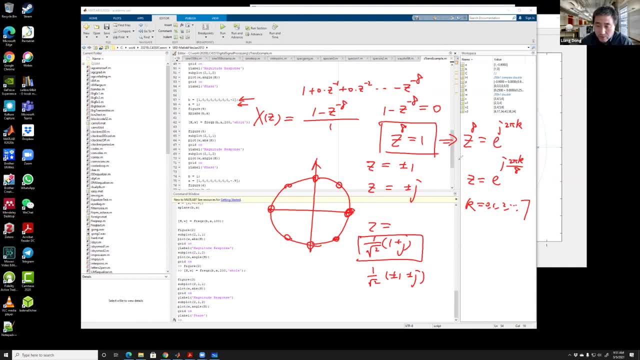 you becomes your original zero. so we have those solutions for those eight numbers again, because z is a complex number, so we need to think in the complex plane, all right, so let's see if this is the case. um from my prompt. so what we have here is um. 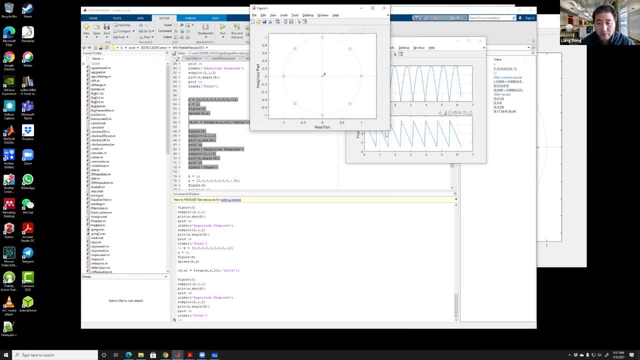 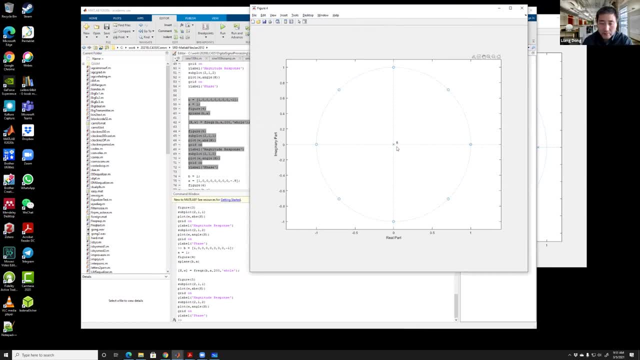 figure four. first figure five. figure four is showing that's a z plane. so indeed it's showing me eight poles on the origin implied and i have eight zeros at the unit circle. now we care about these because when i have a real system i really travel along the unit circle. so it affects me, i'm travel along. 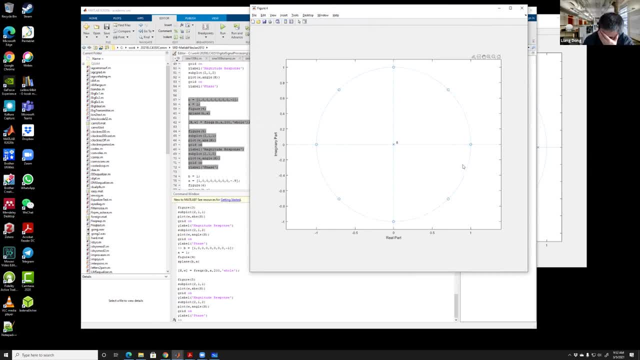 the unit circle, those are eight zeros. so what does that give us? when i check with spectrum in frequency in a practical system in frequency, well then, when you travel along this you will fall to zero. when you start it at dc and then you travel along. here you got this part. this part is your frequency pi over four. 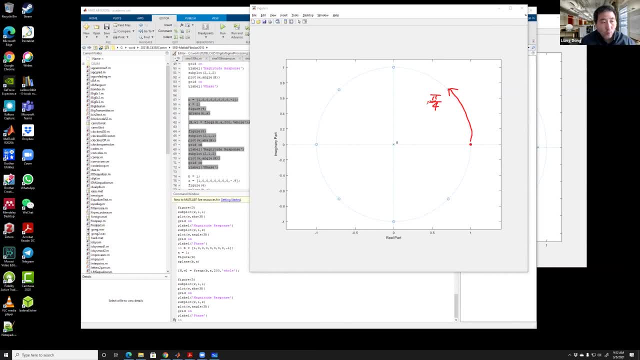 and, of course, we know that you need to somehow map data with your sampling frequency, but digitally, in a digital world, we know that's a frequency power over four, this is a frequency power over two, and when you moved here, that gives you all zeros, so that gives you this. 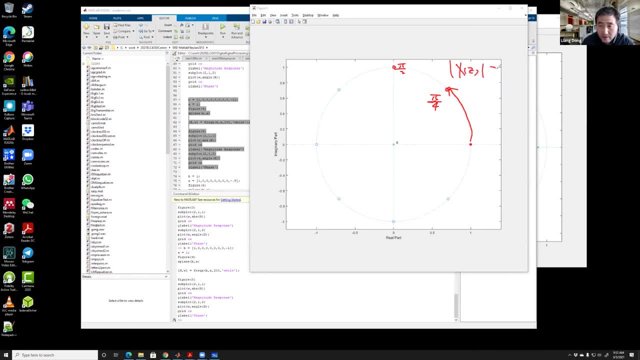 xz or hz, if it's system that gives you this value equal to zero, exactly zero. so that's because you're justあ with the display value. thisienen, you're going to know that it is the same zero, but you have big differences. yes, exactly, on this fine join on these clouds. right there. so, for example, i'm moved to an island of our system- Really change your будong Unter assisting- and i'm moving to a region which is a region called because it's not exactly on this point, on those eight points, right? so i'm doing a frequencies z, so that's. 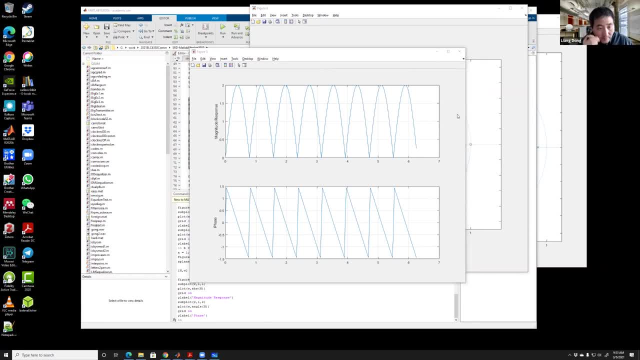 going to show me the magnitude response and face. indeed, a magnitude response is that you know, i have those eight noes, the eight them there, those eight frequency points is exactly move to the zero. so my h, z or xz becomes zero. but if you look at the face, it's actually 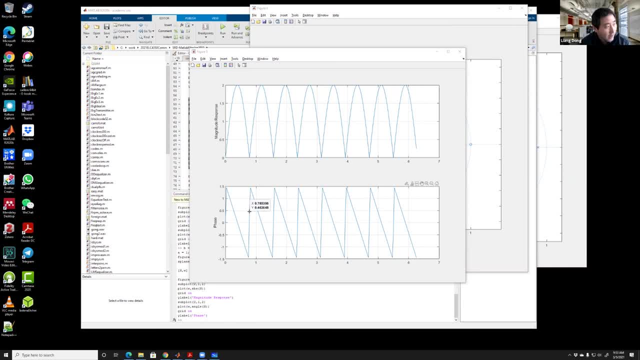 linear phase system because it's an fir system. I only have numerate, I do not have anything on denominator And what you see here is because of the wrap effect. So you wrap around a pile of pi, positive and negative, pi over two. 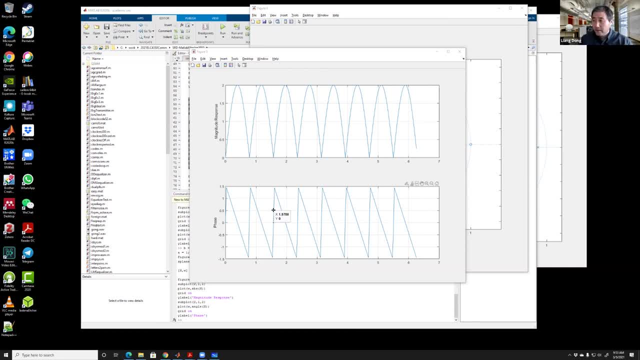 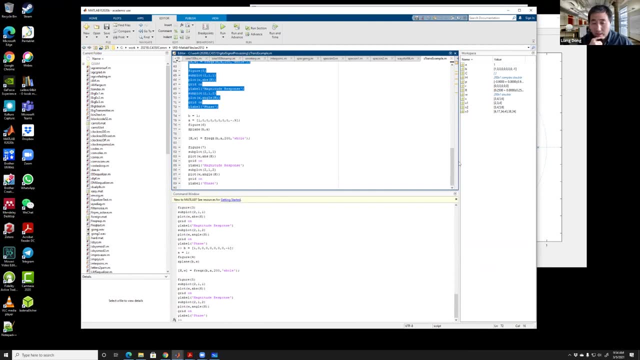 positive and negative, pi over two. So when you connect all these together, it's a straight line, Okay. And lastly, since we play with zeros, let's also look at what about poles. So I the last example I have here is that. 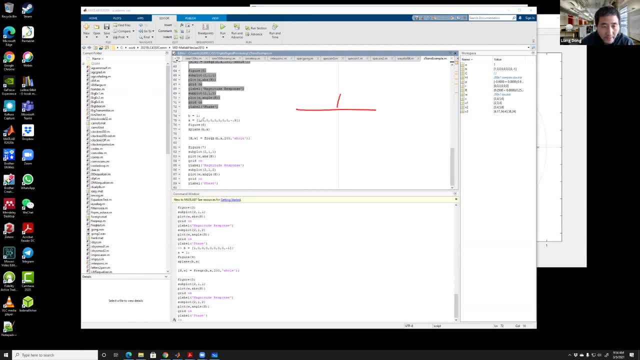 I make a B equal to one, but A is here. If you look at A, this coefficient, or here, what we have here on the denominator is one subtract 0.9 times C to the power of negative eight. Okay, So that's what we have for this function. 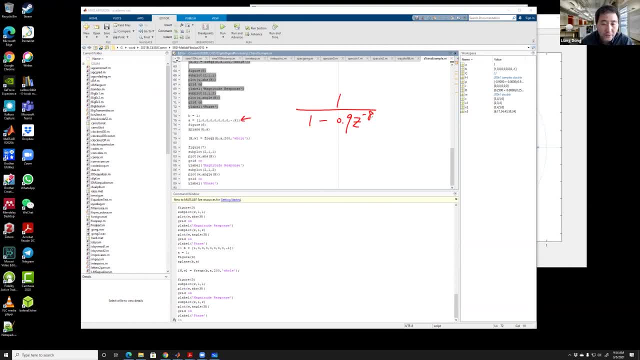 Now I want to make the poles strictly within a circle. Therefore I put a 0.9.. I want to make these all eight poles strictly within a circle. Then, doing the same thing, I plot out the Z-plane, I plot out the frequency, magnitude and the phase. 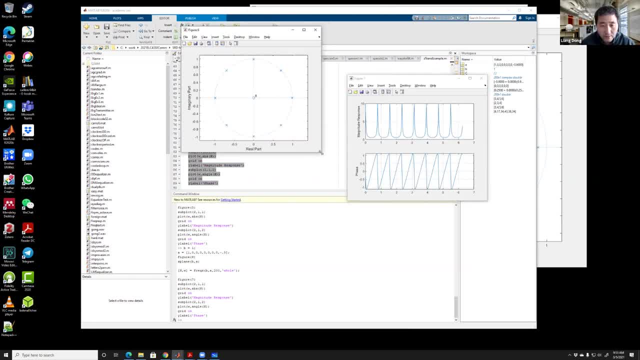 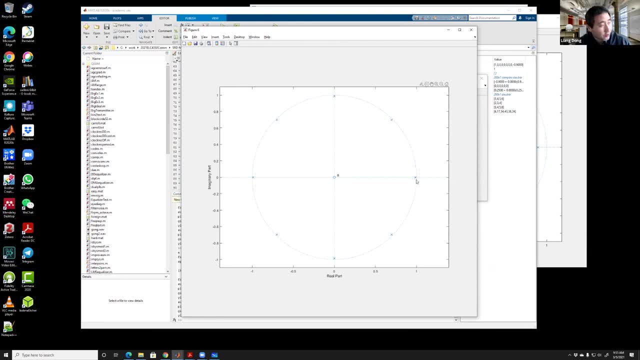 So here is the picture for zero and the poles. I do have eight poles. that's close to unit circle. Remember I put up coefficient 0.9, it's not one. So it's not exactly only in a circle, but it's close to the inner circle. 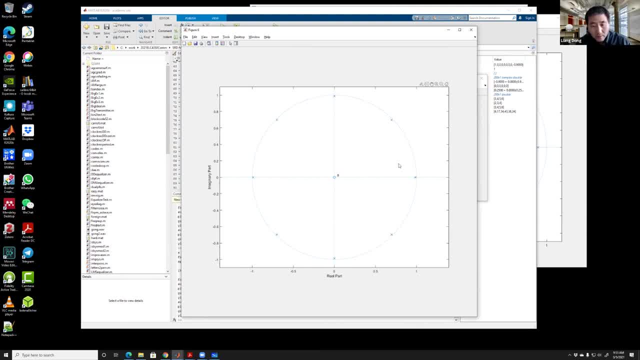 I have exactly those eight poles. Now, when I travel only in a circle, I'm checking frequency. Then if I'm moving close to DC, moving close to frequency of pi over four, I should get that large number because it's close to a pole. 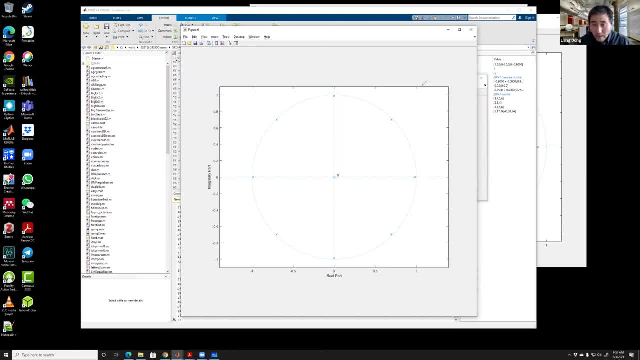 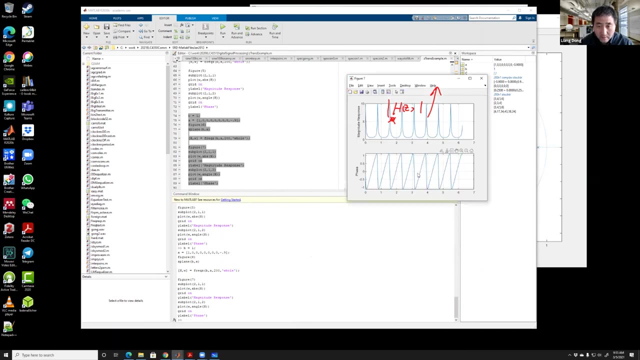 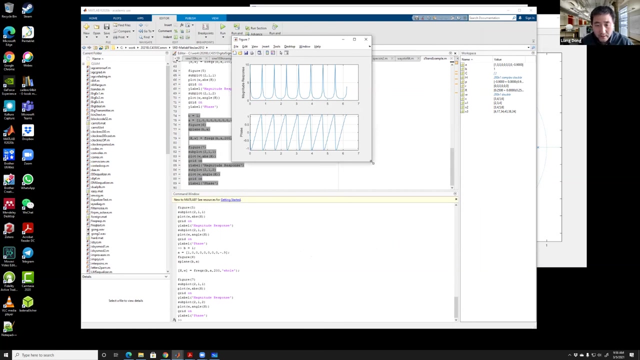 You just simply have this H of Z, this number quite large, And then, lastly, what we see here is the frequency. That's the last picture. So, yes, as we designed, I want to make sure that on those eight frequency positions, 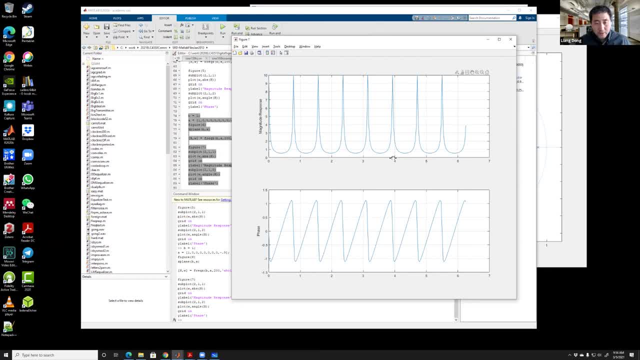 I have a very large magnitude, response of a very large HZ. So indeed this is the case. I got those eight spikes, eight spikes very large, And you can imagine, if I have the poles on unit circle, those spikes will be upward to the sky. 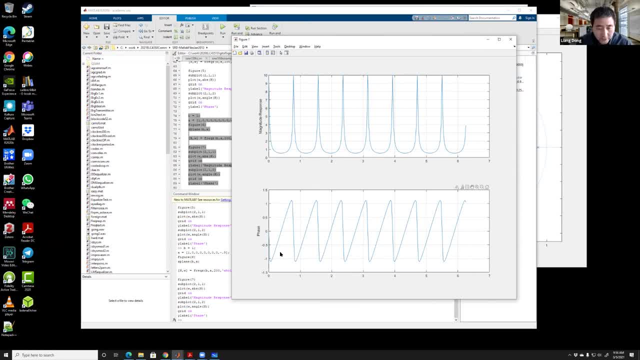 It. just it blew up very large. And then we check the face. This face is a non-linear. They have some of curvature here. It's not a straight line. If you connect, it's not a straight line Because, again, this is an IIR system.